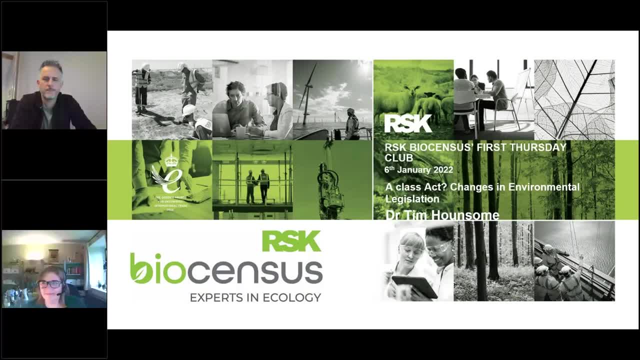 Thank you very much for joining us today for our first Thursday Club of 2022.. I'll just allow a minute or so for a few more people to come in. We've got a huge number of attendees today and people are still joining us, But while we're waiting, I'll just introduce myself. I'm Stephanie. 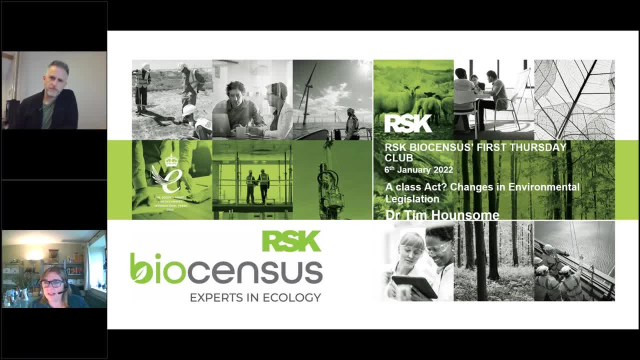 Ray from RSK, and our speaker this morning is Dr Tim Hounsom, who's the Managing Director of RSK, Biosensis, And this morning Tim's going to be talking about a class act changes- environmental legislation relating to the new Environment Act. So thank you all very much for joining us. 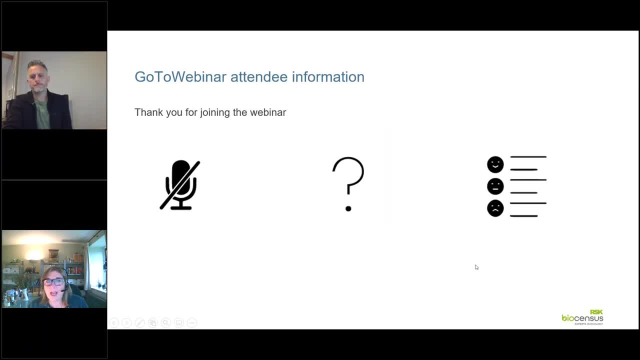 Before we start, we've just got a little bit of housekeeping to do. You'll notice when you join that your microphones are automatically muted and we'll keep them that way throughout the presentation today. If you have questions, then please add them to the questions box and at the 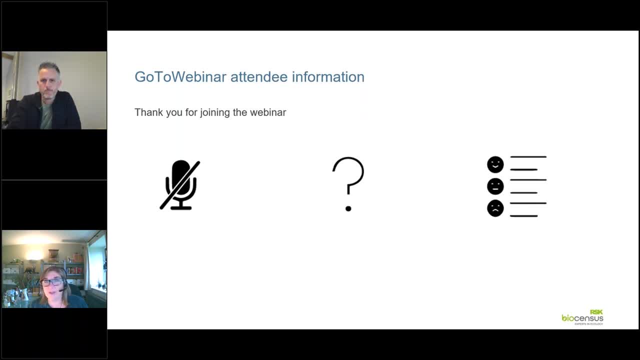 end of the presentation, Tim will answer as many as we can, And if there are some that we can't get to them, we'll try and contact you separately with them. if indeed we know the answers, Shortly after the presentation ends today, you'll receive an email with a short survey. 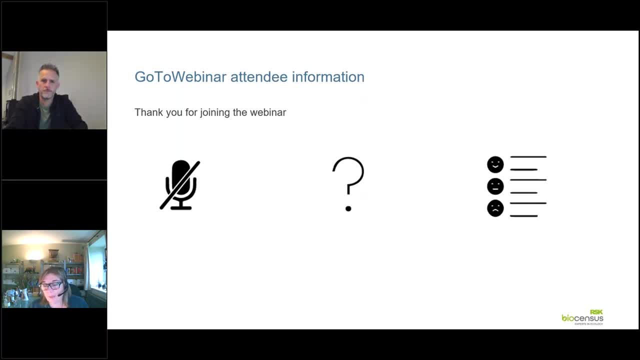 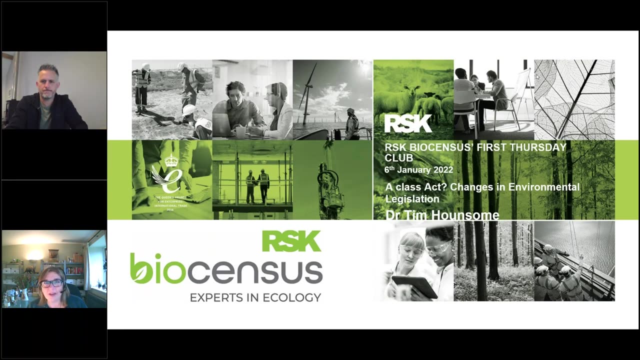 It will only take two or three minutes to complete, and it would be really helpful if you could do that for us, to give us some feedback so that we can help to shape future webinars that we do in this series. So I think we're all about here now, And so, with no further ado, I'm going to hand over to Tim. 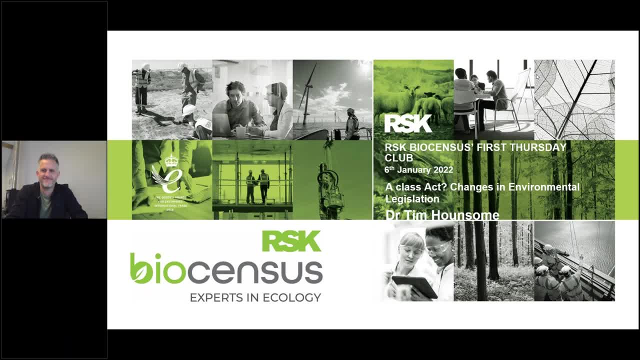 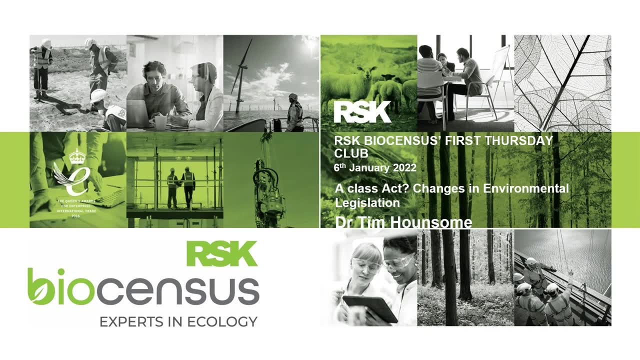 and say thanks very much. Tell us about the Environment Act. Thanks very much, Steph, And hello everybody. I suppose I should also be saying that's the first thing that I'm going to say. I'm going to say: and Happy New Year. It's the first Thursday meeting of 2022.. I was forced to say that. 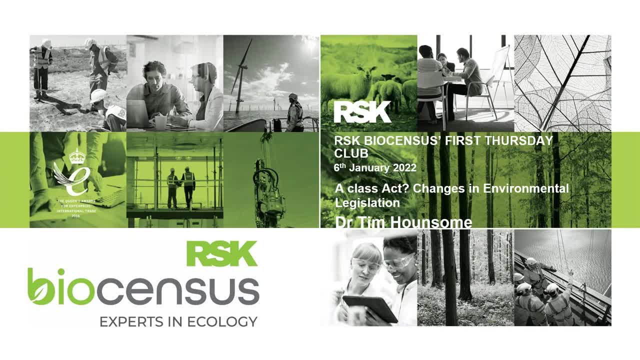 But, as you can see, and as Steph's just said, I'm going to be talking about the Environment Act that came into being as a nice, new, shiny piece of legislation in the environmental sector in the back end of last year. I'm going to start with a disclaimer. 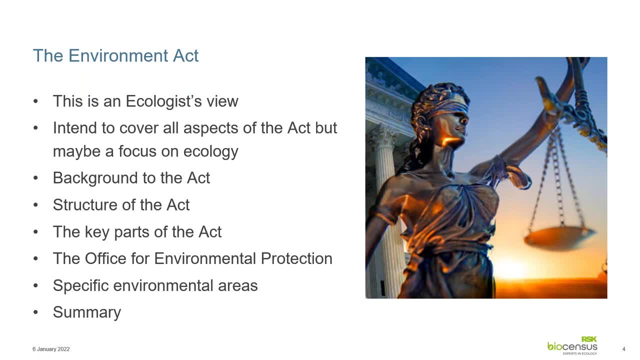 I'm not a lawyer. I haven't helped draft this legislation. I'm an ecologist, and what I'm going to be presenting today is very much an ecologist's view of the Act as it appears. Obviously, I feel sort of duty bound to say that none of this is going to be legal advice. 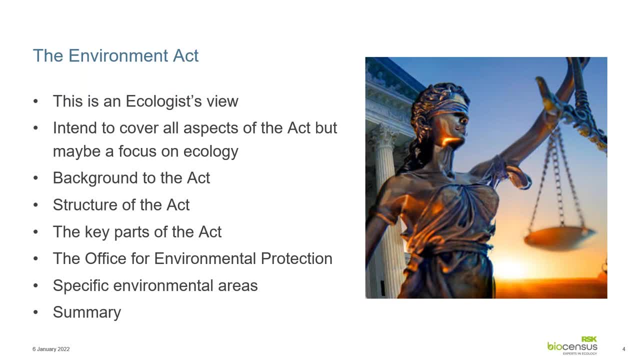 and you certainly wouldn't say that from an ecologist, especially not even an ornithologist. My view on the Environment Act is, and I guess would always be, that I'm an ecological consultant. I run a large ecological consultancy business and I've been in and around conservation and the ecological world my whole career. 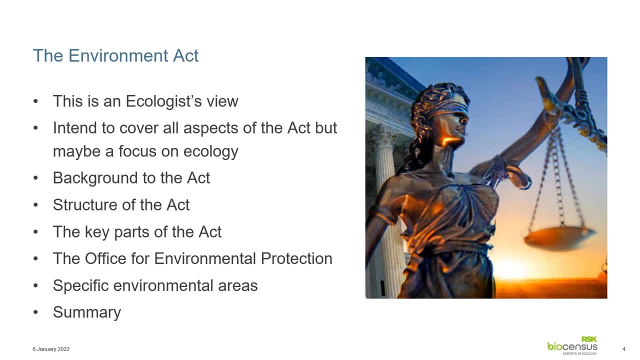 which is longer than I'd want to admit, But let's just say when I started there weren't any mobile phones. Working at night on your own by water was considered safe as long as you could hold your breath, and a little e-grit was something that a twitcher would get out of bed for. 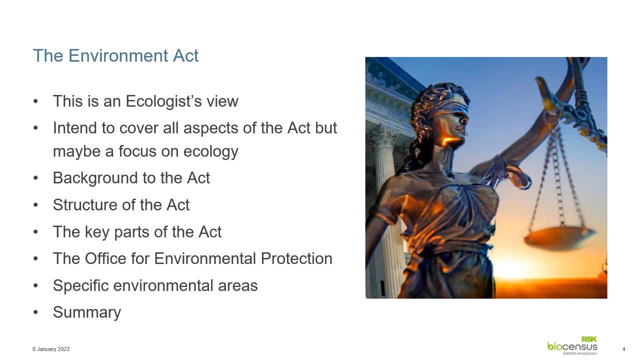 Times have changed. As a result of my career and my work with ecological consultancy world, I've obviously been hugely invested in this subject and I've watched developments keenly for the last few years. What I'll be presenting today is a bit of a background to the Act. 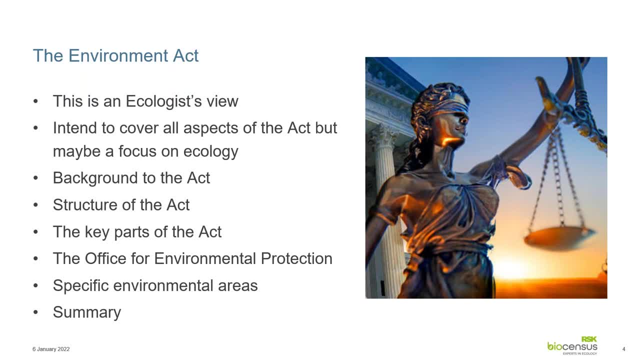 to put it in the historical context of where, why it actually came into being in the first place and why we needed it in my view. I'll then run through the structure of the Act, how it's been laid out, and then I'd like to go into a little bit more detail about how it's been laid out. 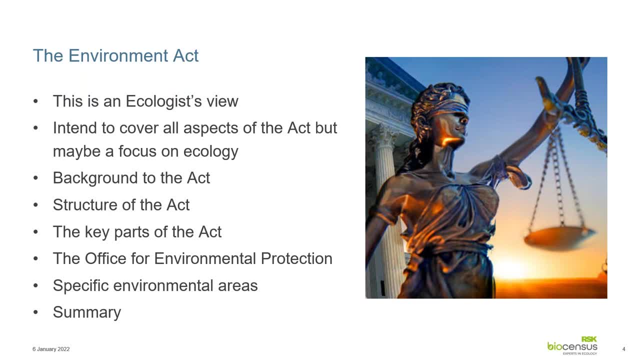 and then I'd like to go into a little bit more detail about how it's been laid out, and then I'd identify the key parts of the Act. Now a bit of a spoiler alert. the first bit is the creation of the Office for Environmental Protection, and obviously I'll talk about that in detail. 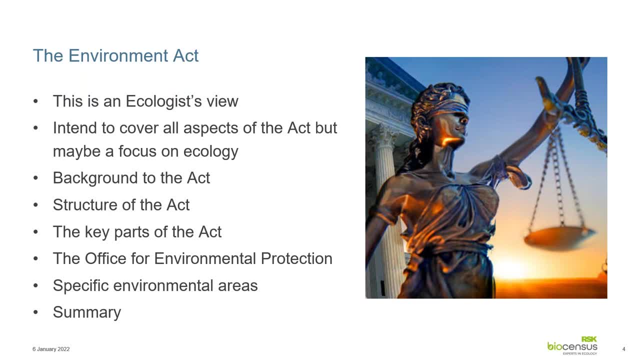 But after that, other parts of the Act deal with specific environmental areas, such as nature and biodiversity or water and so on. so I'll talk about that. But, just to reiterate, I will be pulling out bits of the Act that I think are relevant from. 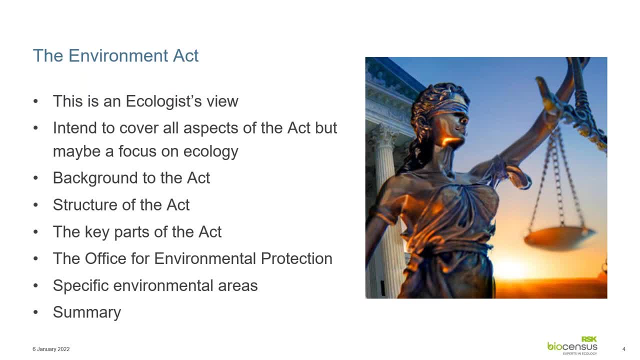 an ecological consultancy point of view, and I hope that you, as an audience will identify certain elements that are relevant to you, and maybe then you can follow up and go and specifically look at those elements in the Act and do your own research. Obviously, then, I'll. 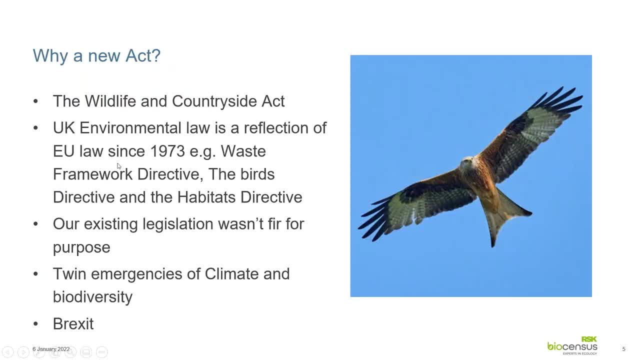 end with a summary. So why a new Act? I think the first thing to do is to put this in historical context, and this is important to understand where we are now. Throughout my career, the influence and presence of the wildlife and countryside. 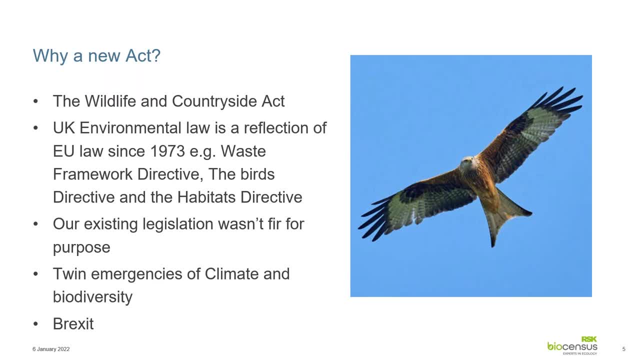 act has been massively influential. this landmark piece of legislation arguably laid the way for the birth of the ecological consultancy sector as we know it. as a result of the wildlife and countryside act, suddenly people, businesses, other entities were legally obliged to do certain things in a certain way, and if they didn't they would be guilty of an offense. obviously this worried them and they went. 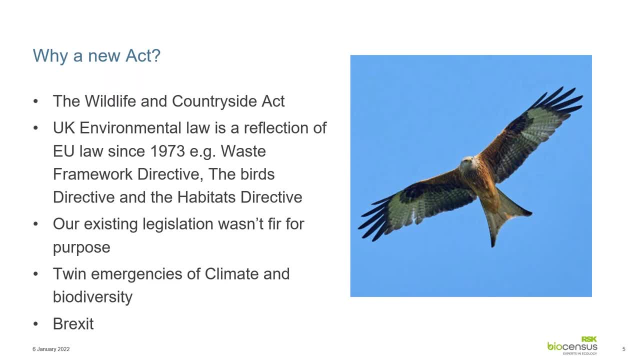 around trying to find people that could help them and, generally speaking, they were looking at naturalists and academics, people that understood how to count butterflies or or identify protected habitats, and gradually, over that time, since since the early 80s, these naturalists and academics have morphed into ecological consultants. i guess you could argue that some more readily than others. 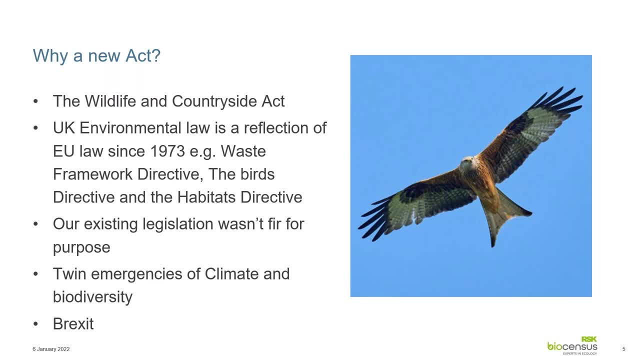 and in fact i know a few that are still morphing. the wildlife and countryside act, of course, wasn't the only legislation that was influencing how species and habitats were protected in the uk, or rather the environment, but the 1970s onwards, the influence of the european union on our environmental law has been profound. 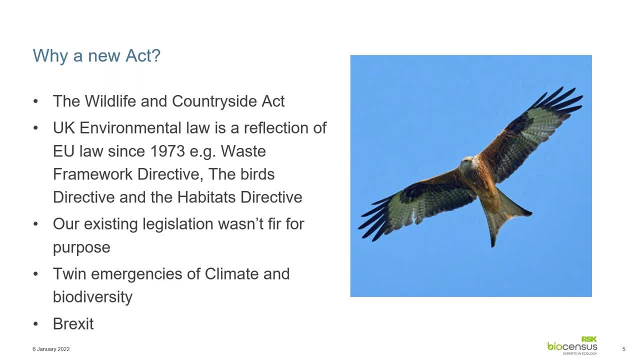 for example, the waste framework directive, the birds directive- obviously, as an ornithologist i was going to mention that one habitats directive, and that's just a name but a few. in addition to the european union's influence on the drafting of uk legislation, it's, of course, been sitting there as a 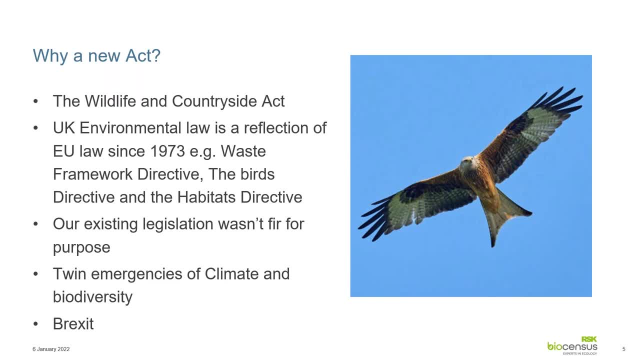 arbitrary iterator as a final decision maker, as the headmaster almost, and so, therefore, most of our case law in the uk is also influenced by the decisions from the european court justice. this, in turn, has had significant influence on the way we go about our work in the environmental consultancy. 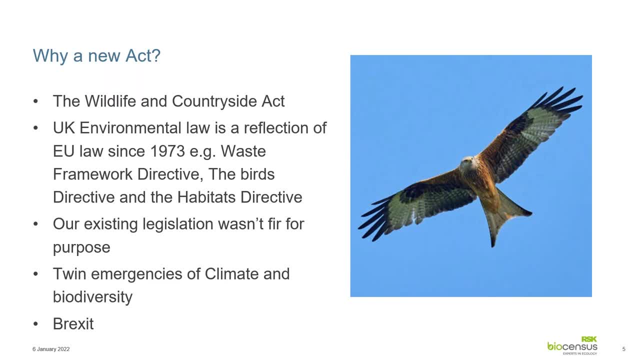 world. i mean, how many times have we said as consultants, or perhaps have heard as a client, that we do things in a certain way because of such and such a case? the example the ecologists often quote is the case from from cheshire, where we were not required to 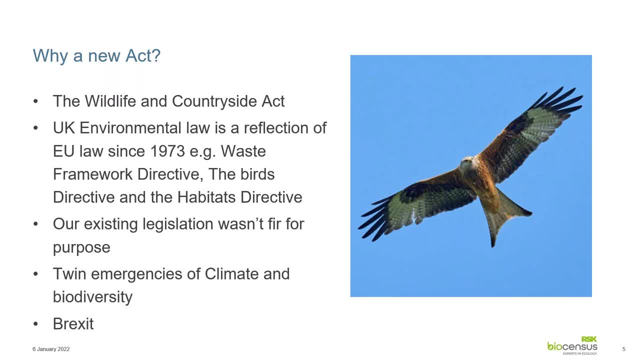 have bat surveys to consent the project. and that was overturned and it was said that in order to consent a project you needed the full information and data before that application could be determined. i think it's fair to say that recently much of our environmental legislation, and certainly our wildlife protection, is starting to feel, if not appear, not quite fit for purpose a bit. 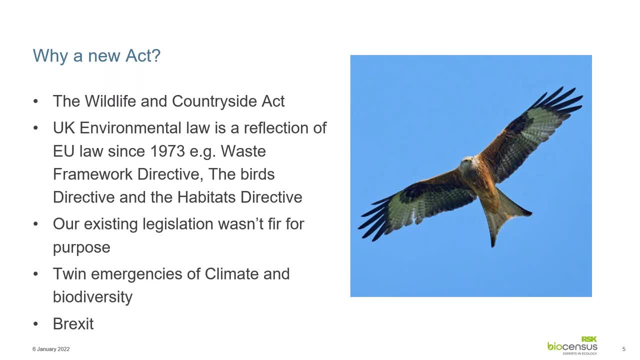 a bit tatty, a bit tatty. can you talk? a little bit younger of me? yeah, so i think, um, you've got to say a bit about the implications of those indices. i think they're very. these are some of the solutions for us when we work from home. 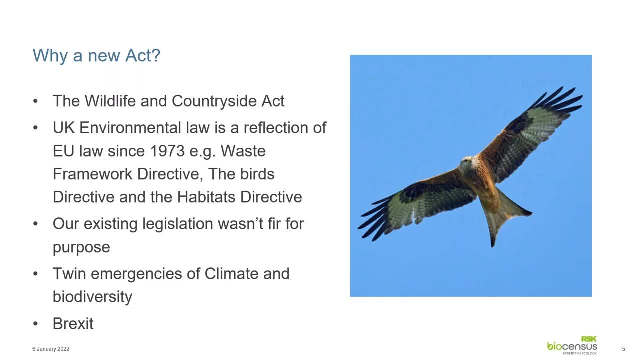 but i do think the navies are very positive words, so there's a bunch of ways that we can put them in place for that reason. but i think it's something i'm kind of curious about. when we talk about I'm a bit too political and it's hard to talk about an act of Parliament without having 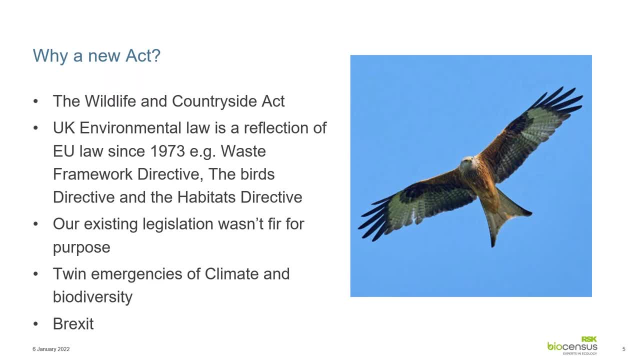 a political slant on things. so forgive me, but I do feel that, however well-meaning and however much passion and science and political will to change and avert these situations that was applied, our track record in this field is rubbish On our watch things have. 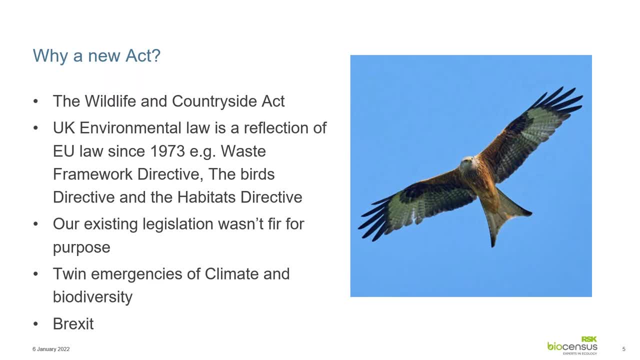 got dramatically worse. However, over the last few years I've been encouraged and I think there has been a clear and obvious step change in where the environment sits on everybody agendas. I mean not just conservation and environmentalists, but politicians, the man. 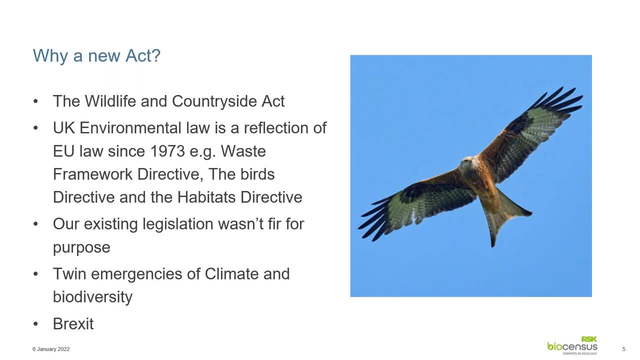 in the street, people that are now aware of things like biodiversity and environmental damage and climate change. I think probably at the moment, arguably, it's only second to COVID in everybody's agendas, And you know, speaking as a conservationist and environmentalist, 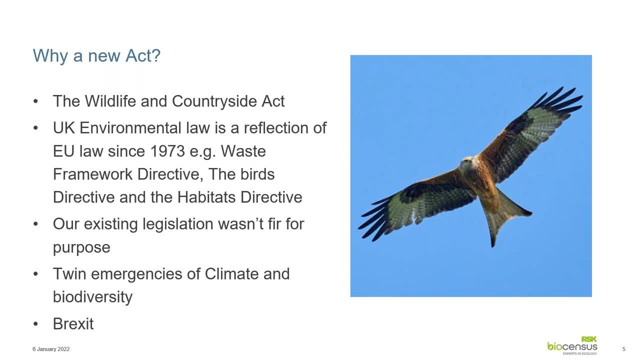 this is great news. you know about bloody time. Let's just hope it's not too late, I guess. And finally, the penny is dropping. So, looking specifically at the UK, whatever the legislation the UK or the European Union derived and legislated for obviously hasn't worked. The 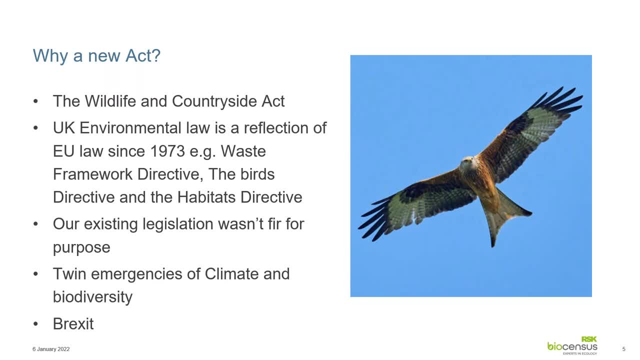 Farmland Bird Index shows dramatic falls in species and abundance. Many, if not most, of our rivers are polluted. the air quality in places in the country is worse than it ever was. Effluent discharge from water treatment works is at critical levels. As much good. 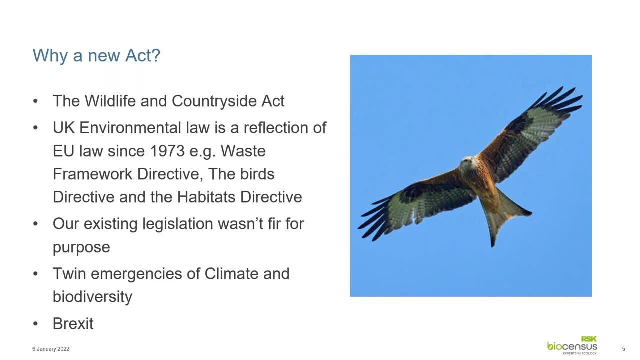 our laws have done. they simply haven't done enough. That sounds quite negative. I realise that. but here we are with this underperforming and not fit for purpose statute book, a twin global crisis of climate change and extinction rates, and at the same time we're walking. 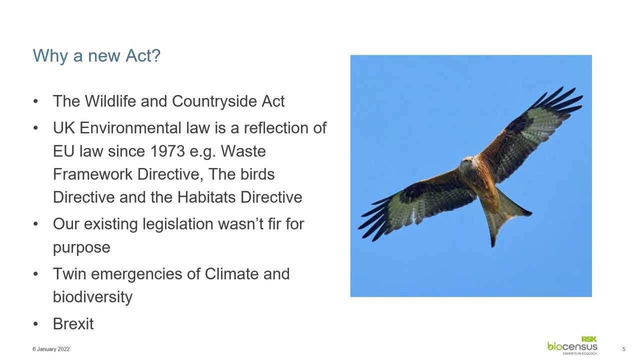 away from the organisation that has given us much of our environmental legislation and, even more critically, held us and our governments importantly to account. One might see this in a doom and gloom way. many do, I can assure you, or you could see this as a perfect storm. 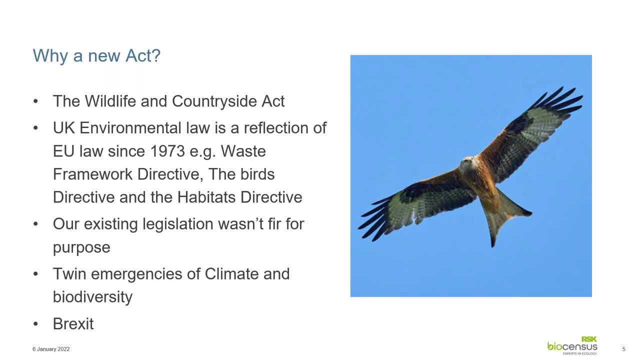 as a once in a lifetime opportunity to get ahead of the game. Personally- and if you'll forgive me, I think I'm in both camps. I will always remain cynical of politicians and politics. I think that's a healthy place to be And the UK government not being held to account. 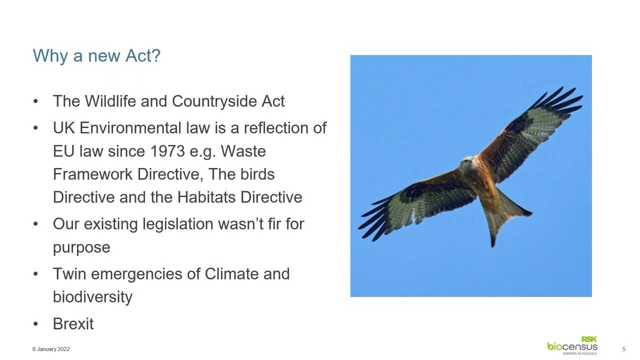 by a higher authority such as the European Court really worries me, And I think that there's a lot of other reasons why this doesn't happen to us. We'll all agree that this is not a good time for politics, but it does get close to it as it. 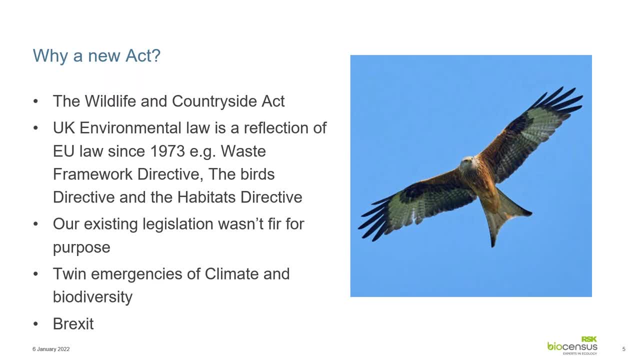 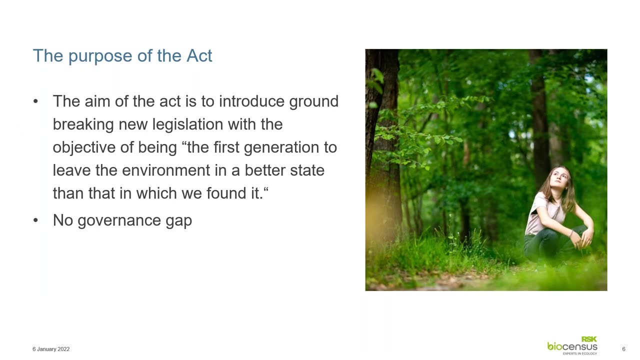 does many others. But on the flip side, I think I will also admit to a certain sense of freedom and opportunity that this gives us as a nation. We now have the opportunity to draft and enact legislation. that means that it paved the way for us tackling once and for all the way we use and interact and leave our environment. 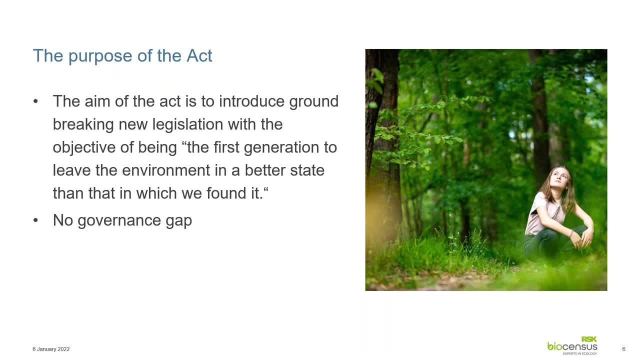 we are indebted to Mr Gove for some of the initial influence here. In the preamble to the Act itself, it states that the aim of the Act is to introduce groundbreaking new legislation with the objective of being the first generation to leave the environment in a better state than in which it was found. 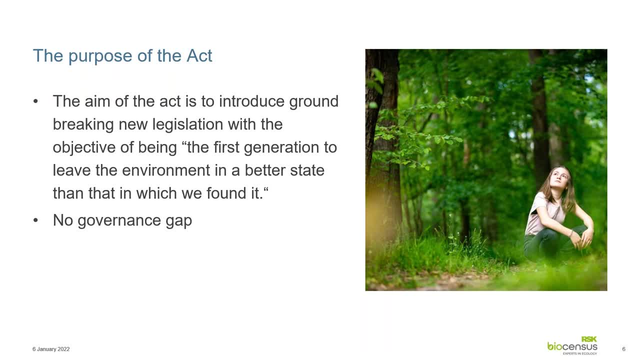 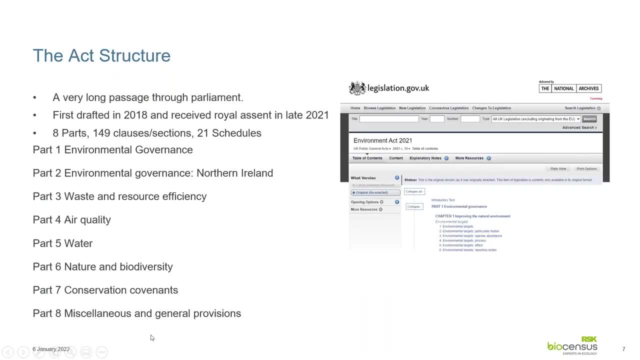 There was also this tacit reference to Brexit, with an express purpose of ensuring there was no environmental governance gap. So that's the background. What is the Environment Act and what does it cover? First thing to say is that, in order to pull all this information together for today, I'm 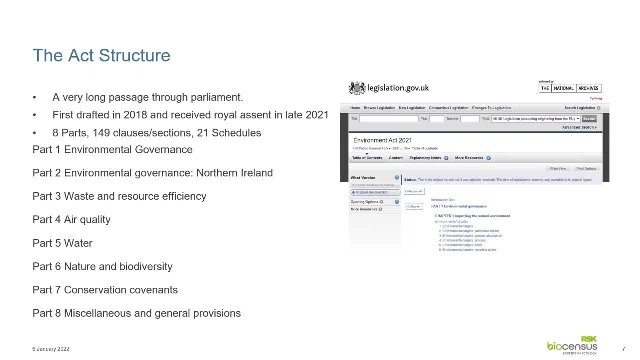 indebted to a host of articles, websites, etc. My intention isn't to go through the Act line by line- collective side relief- but to pull out key points, And I will say again, key points to me as an ecological consultant, which hopefully 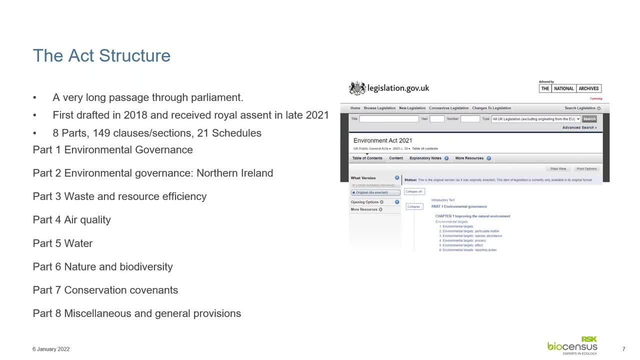 will resonate with you. This isn't supposed to be a full analysis of the Act, So some facts about the Act itself. I mean it had a very long, protracted journey through Parliament. It took over three years from its initial conception in 2018 and to get its royal assent. 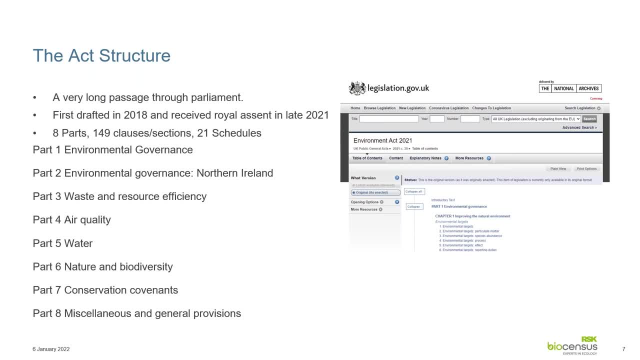 in the back end of last year. I guess to a certain extent it's just probably influenced by COVID, But I think also it was a heavily debated and contentious bill, and quite rightly. And so I think. as we talk, as I go through my talk, you'll see 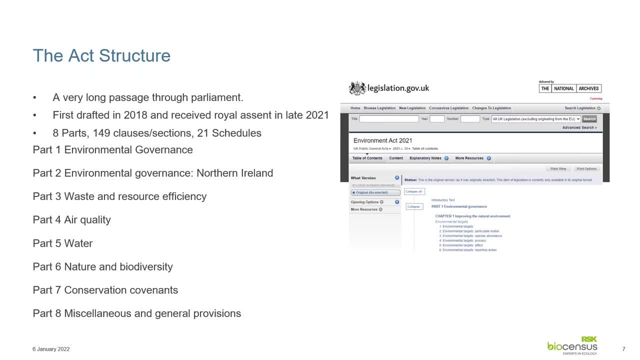 There's a lot of elements of amendments that were tabled that have actually strengthened the Act. as it turns out, It went through three parliamentary sessions and was in two Queen's speeches. Just quickly look at the structure of the Act. deceptively simple as all these things. 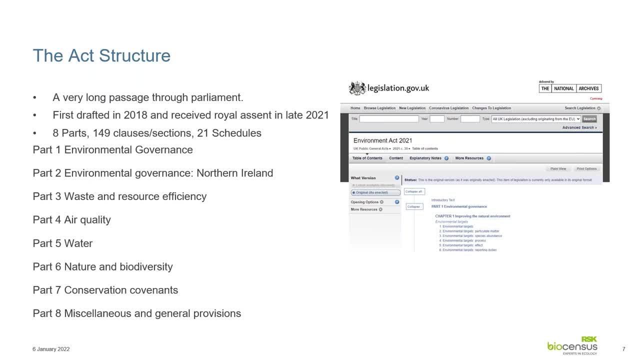 always are. It's laid out in eight parts. There was 149 clauses and sections within the Act, And then at the end there was 21 schedules, So there's a lot of things that are appended to that. What I'm going to do now is go through these various parts, although I will be missing out. 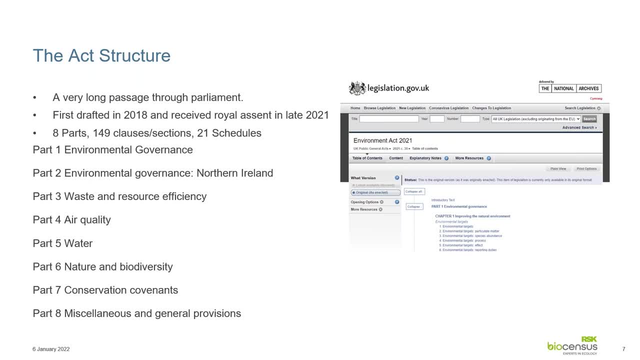 a couple. The first point I'd like to make is I'm not going to be talking about Northern Ireland in this particular case, I think. as far as I understand it, currently it still hasn't been passed through the Assembly, And the miscellaneous is what it sounds like. 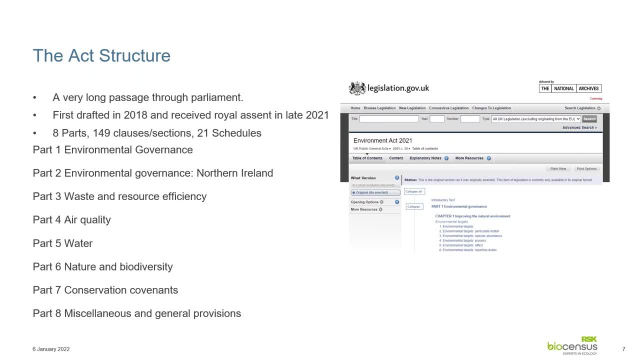 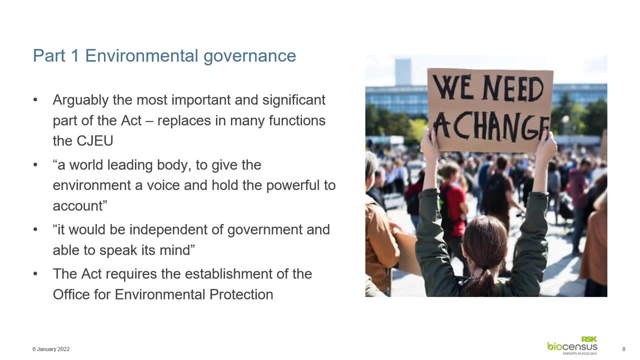 And I'm not going to be talking about that today. OK, Let's talk about part one: environmental governance. For reasons I've already mentioned, this is a critical part of the Act. I don't think I can underestimate how important this bit was, considering what was happening. 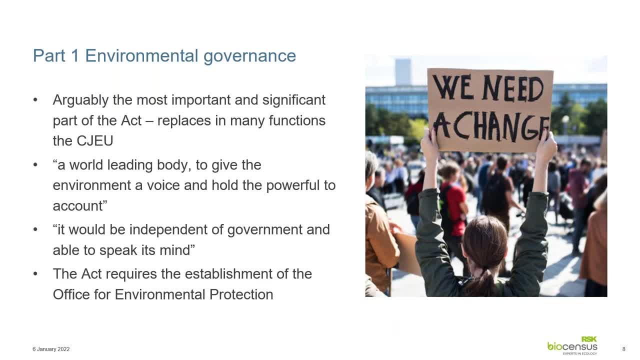 with regards to Brexit and so on. So with no higher authority to answer to apart from, arguably, the people or the electorate, it's always been crucial that the Act set out how this would be achieved, how the absence of the European courts would be dealt with. 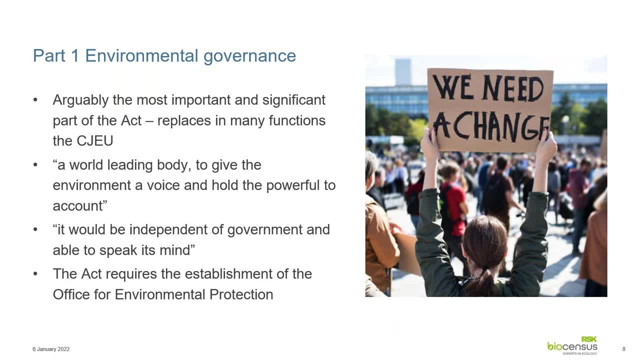 And again we have Mr Gove to thank for some initial statements that set the tone. He said that he wanted a world-leading body to give the environment a voice and hold the powerful to account and, furthermore, that it would be independent of government. and 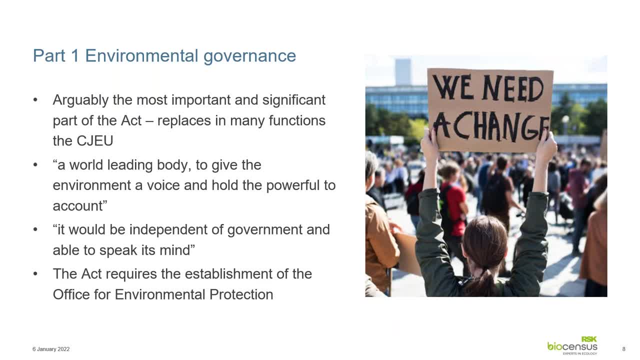 able to speak its mind. I don't think anybody can argue with that at this stage. I think that's a critical part of this organisation. A key element of the Act is the requirement to establish the Office of Environmental Protection, or the OEP. 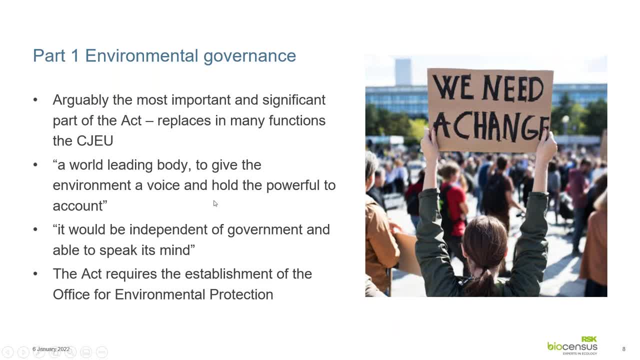 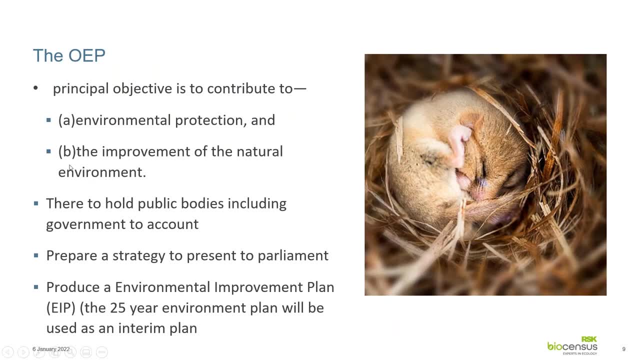 The political rhetoric around this Act has been concerned very much with its remit, the powers that it holds, how it's funded, how independent it's going to be. It has stated that its principal objective is to contribute to environmental protection and the improvement of the natural environment. 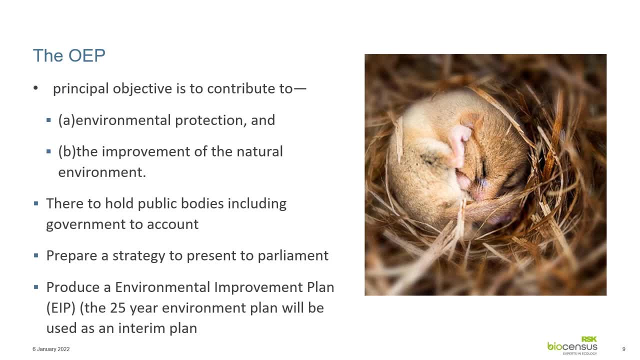 Although the word contribute might sound a bit weak to some- as opposed to enforce or to ensure, in theory, the OEP has the ability to hold anyone to account, including public bodies and, in theory, government. Many consider its ability to do the latter as a critical power when replacing the role. 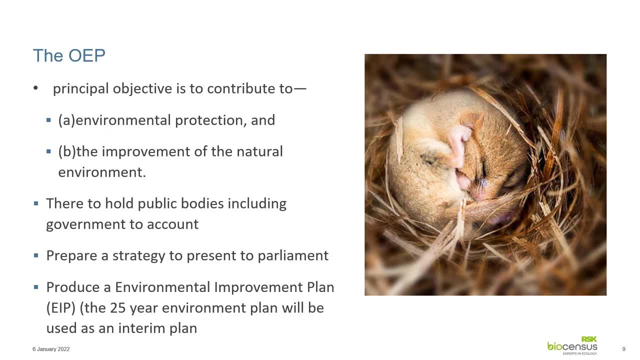 of the European courts. There has been some debate around whether the differing levels of evidence needed to uphold an accusation of non-compliance are relevant. Under EU rules, a state had to have made, or been found to have made, a manifest statement. 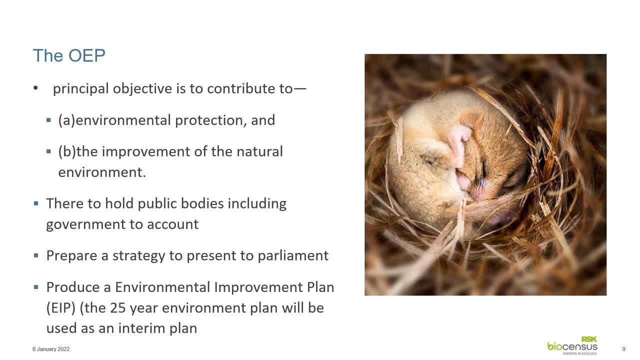 There has been a manifest error in this assessment. From now on, we will almost certainly now rely on judicial review, and many commentators have suggested that this approach is less evidential and therefore perhaps arguably weaker. as a result, The OEP can receive and investigate complaints of serious breaches of environmental law by 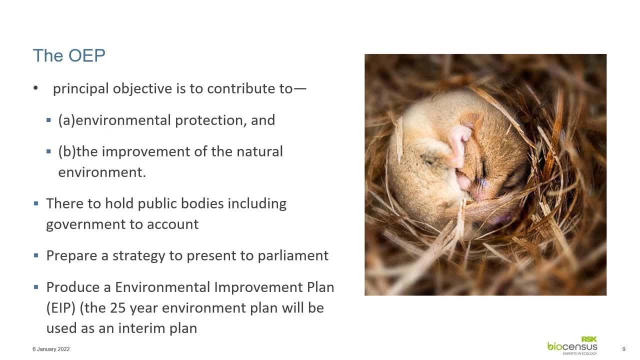 public authorities, including local authorities, government departments and arm's length bodies, And it can also take legal action if necessary. After its establishment, its first job is to prepare a strategy that will be presented to Parliament, and the OEP will also advise on changes to environmental law or other matters. 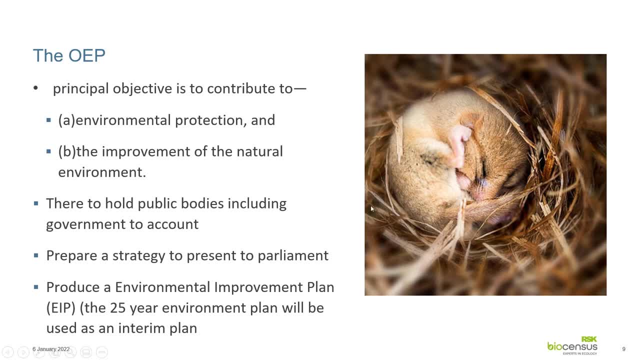 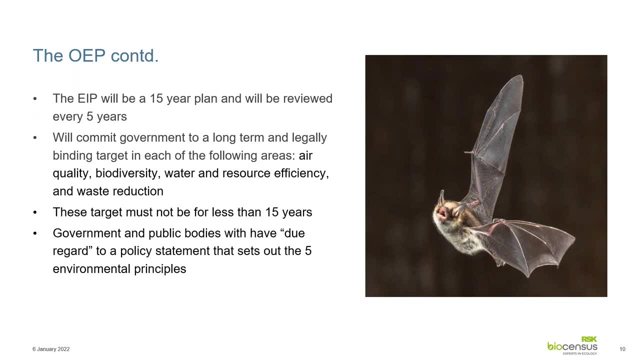 relating to the natural environment. when requested by the minister, The OEP will be required to draft an Environmental Improvement Plan, or EIP. Currently, the 25-year Environment Plan from DEFRA will be used as an interim improvement plan, But then subsequently all EIPs will be reviewed every five years and with each one setting. 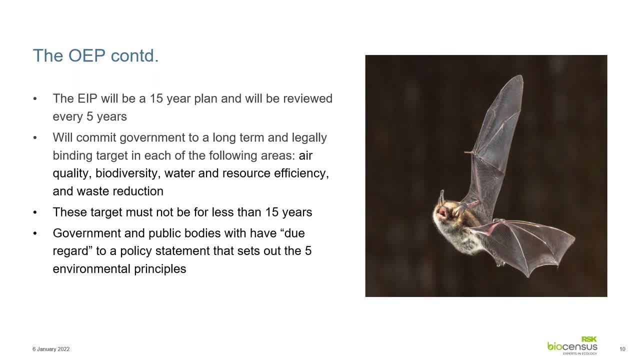 out a 15-year Improvement Plan. I'd like to point out at this point that the longevity of some of these targets is significant and it runs throughout the rhetoric within the Act. I think, speaking for somebody that used to work in the civil service, that this is encouraging. 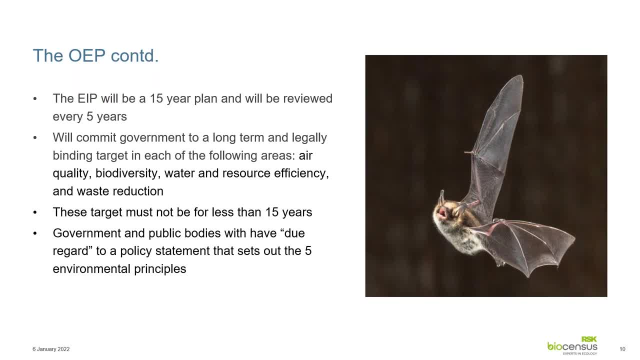 It could be considered as kicking into the long grass, But I think actually It's an acknowledgement that the solution to this isn't in the life of a parliament or in the life of a government. It's not three or four or five years. 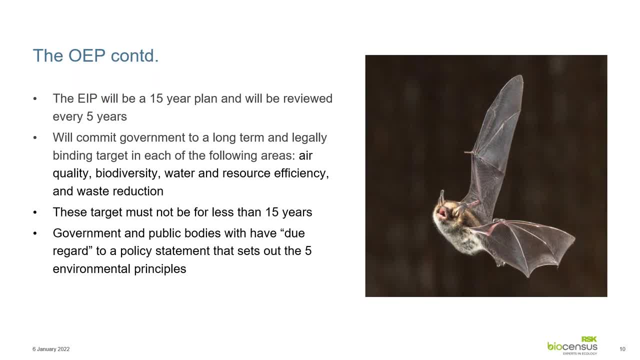 It's not somebody coming in to make a big splash to solve the problem, that this has to be the long-term view. So I'll give them the benefit of the doubt on this. But you will see as we go through this that this is a common thread. 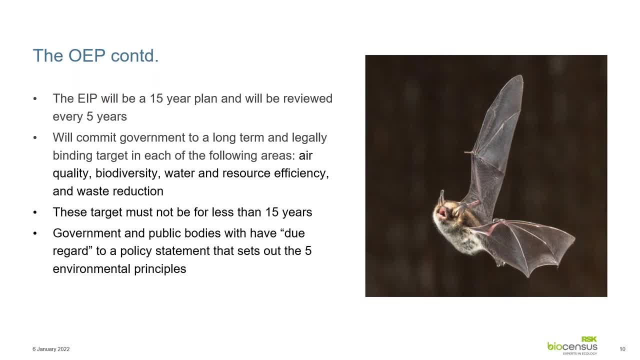 This commits the government to setting at least one new long-term binding target in each of the four areas: Equality, Biodiversity, Water and resource efficiency and waste reduction. The Secretary of State must compile monitoring data to show whether the environment is improving in accordance with the EIP and the progress towards those targets. 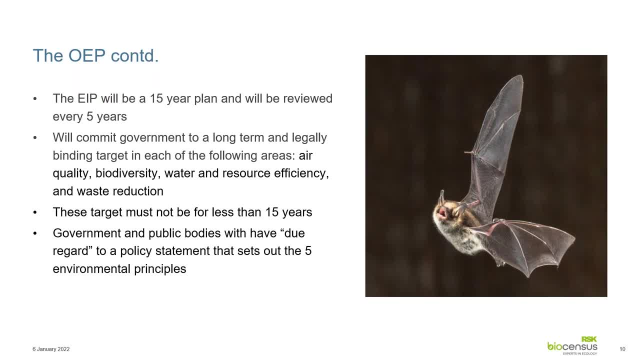 It must also report annually to Parliament on the progress of implementing the EIP. Part of this plan will set these targets, but they will have targets of no less than 15 years. Again, this is the longevity I was talking about. The theory, I guess, is to reassure people. 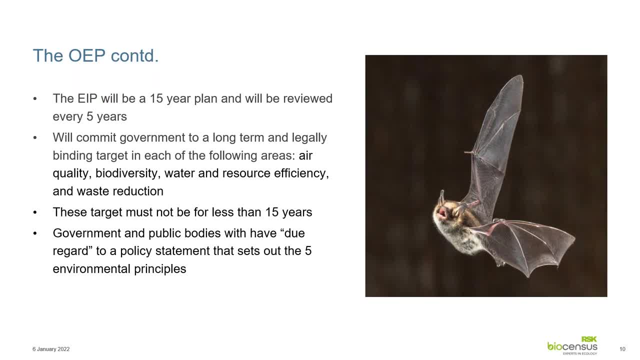 I don't know. I don't know. There isn't much evidence on this now. There isn't much evidence on this now. They might now have a longer view than is normally applied in Westminster. They can, however, set interim targets, but there will be no obligation to meet these. 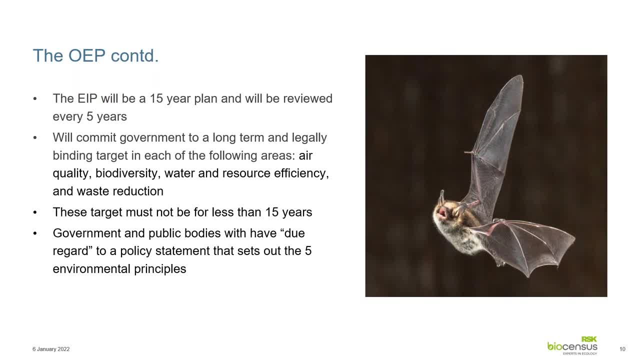 This is the first in my head. This isn't the first slight alarm bell, But I'm going to go in with an open mind. I guess Government ministers and public authorities will have a duty to have due regard to a policy statement which will set out the five environmental principles in more detail. 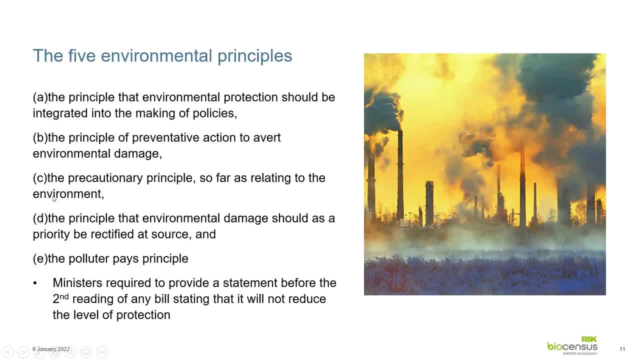 These principles will cover the principle that environmental protection should be integrated into the making of policies, the principle of preventative action to avert environmental damage, the precautionary principle so far as relating to the environment, the principle that environmental damage should, as a priority, be rectified at source and the polluter pays. 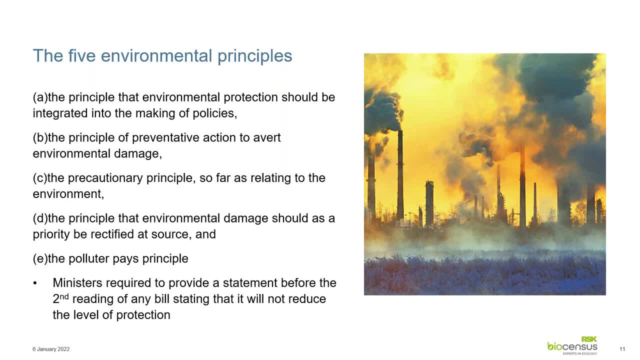 principle. Those of you that have been working in the environmental sector for the last 20 odd years will recognise some of the words within this. based on some of the EU directives and case law, The bill also requires ministers to publish a statement before the second reading of any 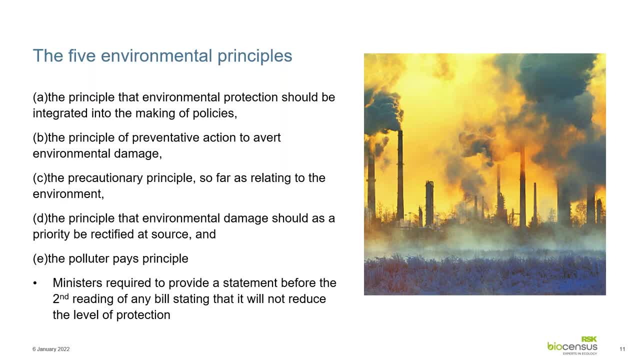 bill that contains environmental law provisions and to state that, in the minister's view, the bill will not have the effect of reducing the level of protection provided by any existing environmental law. The minister's view. Interestingly, there has been some movement on this. 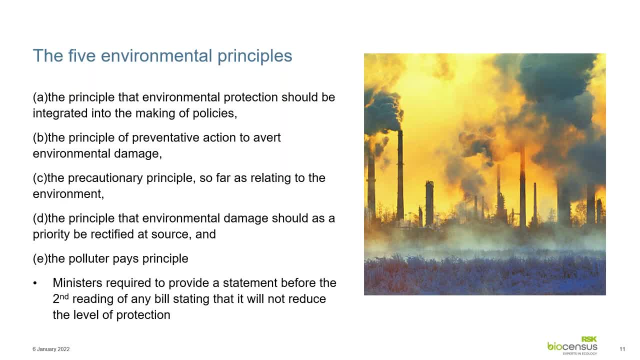 During the drafting, with changes in language, as you can imagine, there was two significant ones here that were removals of clauses that said that the principle would only apply if they were not relevant to policies. Also, if applying the environmental principles to making, developing or revising the policies, 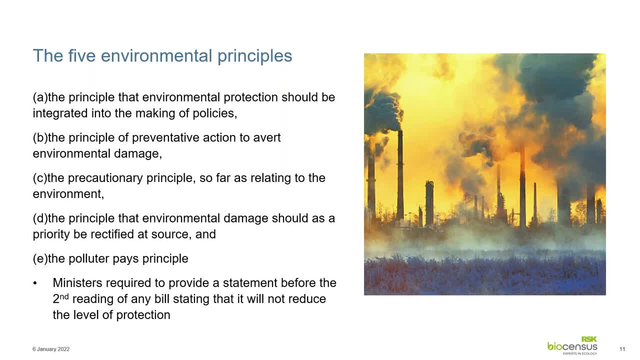 would have no significant effect on environmental benefit. Remember, these were removed. And then there was this actual that sort of if all else fails, we can. we can get out of jail, and the clause again was removed, which was that they don't apply if any other matter specified in regulations made by. 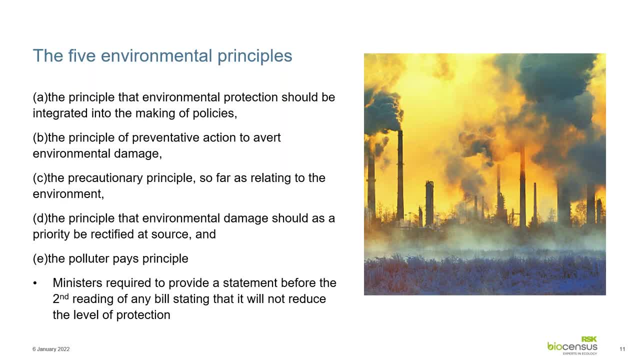 the secretary of state. so, i think, important omissions and removals. just before we move on, though, there is an important point here, which is that the there is exemptions um under this, um the jurisdiction, and that is for the ministry of defense and the treasury, um. i guess you can see reasons why, potentially the mod. 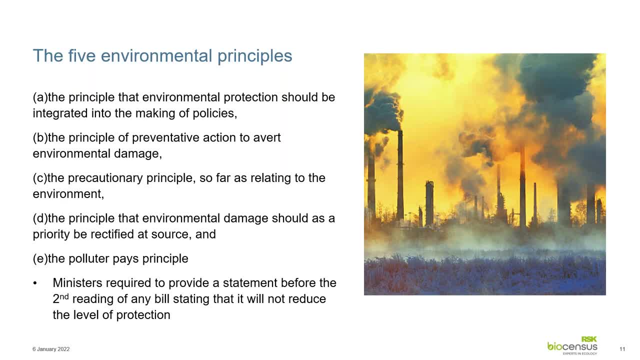 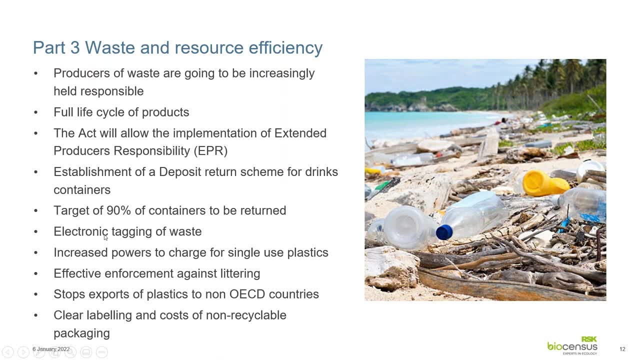 i'm less sure about the treasury and i think we should be watching that carefully over the over the coming years. okay, so that was part one of the act, which covers the office of environmental protection. i've skipped part two because that was, if you remember, to do with. 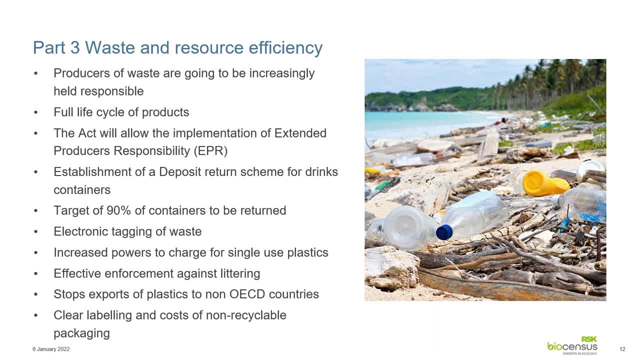 northern ireland went to part three, which is to do with the waste and resource efficiency. the main point here, i think, is a truly significant step change in the emphasis. before the waste was the problem with consumers, but the emphasis here is very much placed on the fact that the issue is with the producers. 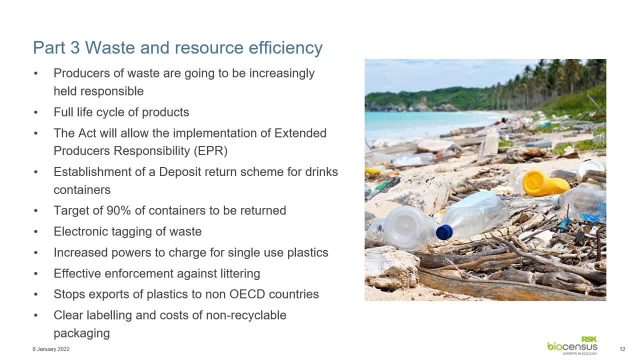 it would appear, on the face of it, that the act will force manufacturers to take responsibility for the full life cycle of the products they produce. powers derived through the act will allow for extended producers responsibility, or epr, to allow the current 10 percent that is currently. 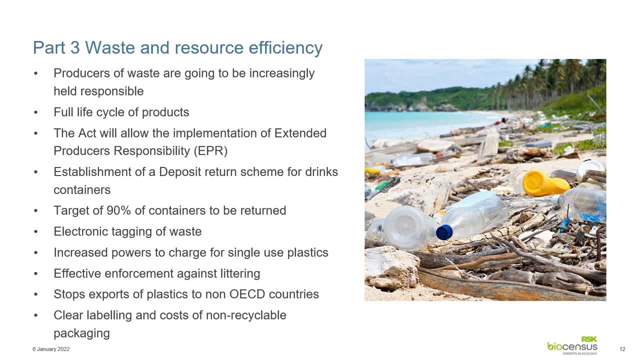 in the areas where there are other existing in the area in which the product is published, although these auctions can be done by separate parties who have been working with different industries in other countries. um. so these are the real set of requirements that we're trying to address. um, the first requirement is that the product be supported by the employers. 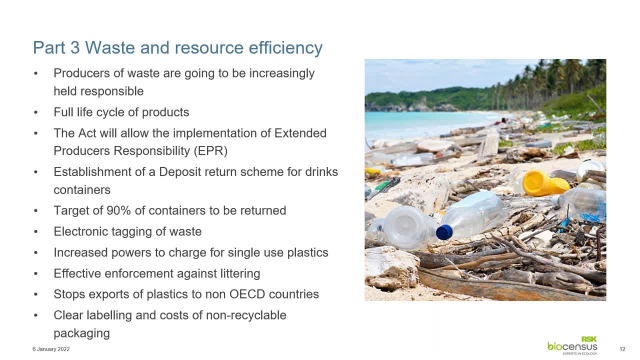 there's also a point on the way that the ill effect. this is precisely the same, as we've said with the previous comments. so that is really important: who are the producers are in the stores and who are the consumers and what their durations will be. so, first of all, i just want to say that the 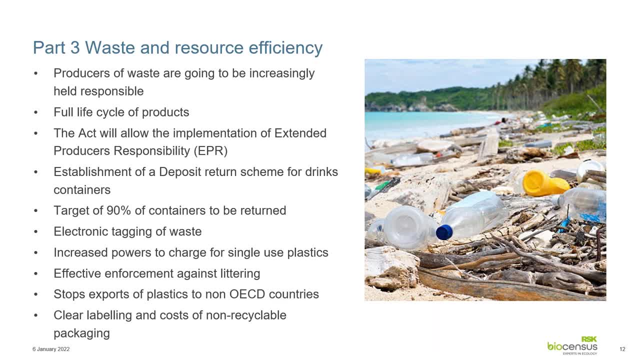 90% of all drinks containers to be collected by the scheme. Retailers who sell drinks containers covered by the DRS will be required to ensure that the deposit price is added to the purchase price and to accept all DRS containers returned to their store. They will need to host a return point, such as a reverse 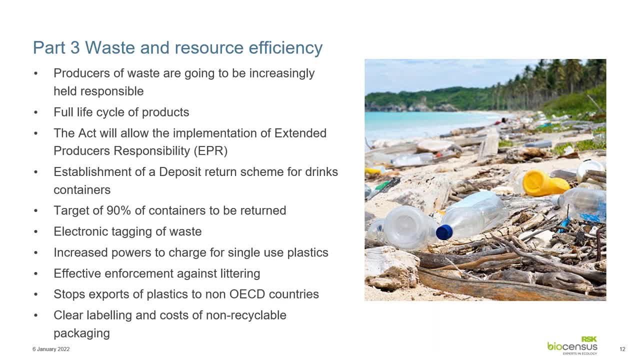 vending machine- it sounds like it's out of Douglas Adams book- or a manual return point. This will be paid for via a handling fee to the DMO. Another clause allows for mandatory tagging of waste or electronic tagging. This will replace this slightly archaic system of waste transfer notices that are sporadically. 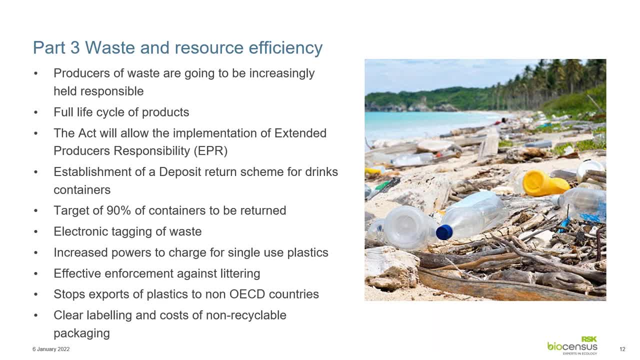 followed up. There will be increased powers to charge for single-use plastics, as well as proportionate and effective enforcement against littering, Although I'm not really quite sure how that would work and I can only imagine. most importantly, the Act introduces powers to stop the exports of plastics. 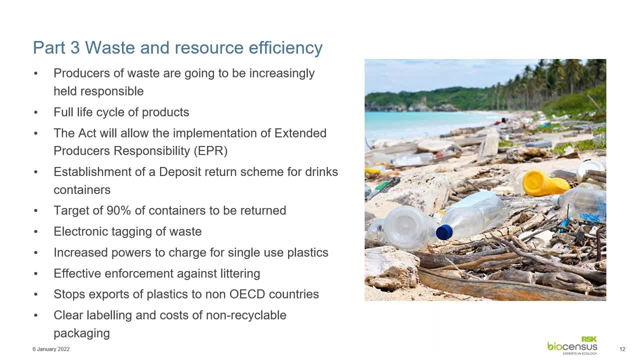 to non-OECD countries, something I personally think has been shameful of us in the past. Manufacturers produce unrecyclable packaging will have to pay higher fees. In addition, producers will have to clearly label packaging. The current estimate of the extra cost of packages is likely to be more than three. 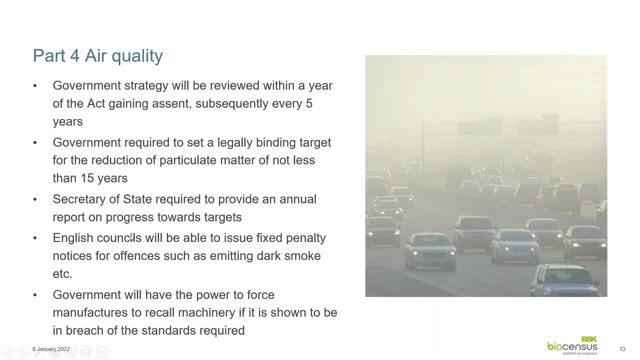 billion pounds. Part four deals with with air quality. These are the main factors. The structure of the air quality strategy will not be as simple as the San Antonioさん's definition of air quality. The new Air Quality Strategy will includeающ스리스와인�전�θ자피� 1990. 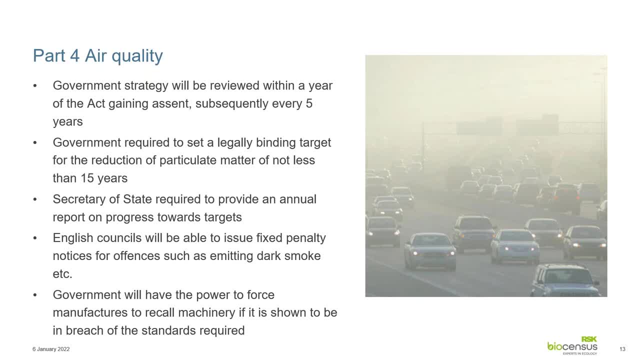 according to the current legislation And the safety of air quality standards, Bioreponse leads to a pretty significant increase in the cost of air quality delivery and its value. This will be released in New York City approaches and employers will be over to TVB on the physicians and, I think, to the 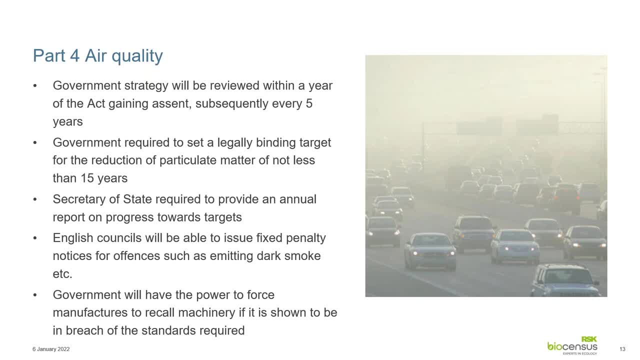 project quanto a week in October 2022, the company that will be working with- and as yet unspecified- air quality target set for at least 15 years in the future. number again three amendments to the Clean Air Act of 1993, English councils and they'll be able to issue fixed penalty notices for breaches with. 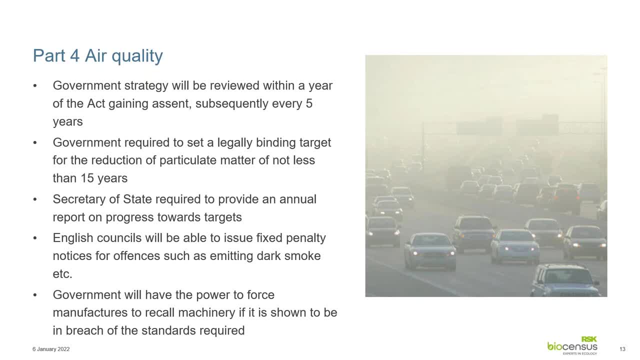 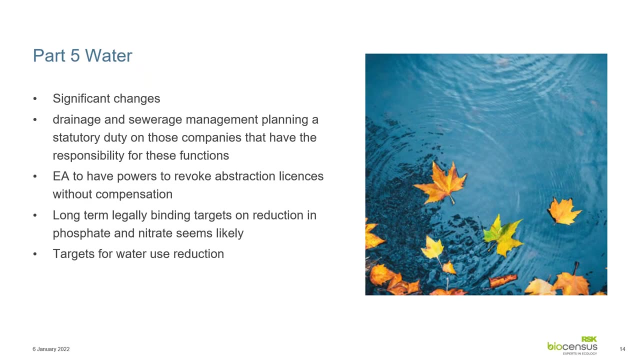 fines between 175 and 300 pounds. the act also empowers the government in order to be able to order vehicle manufacturers to recall non-compliant machinery. part 5 covers all things wet in water. there are some fundamental changes, isn't it, in this area, and it's arguably one of the most significant victories of the. 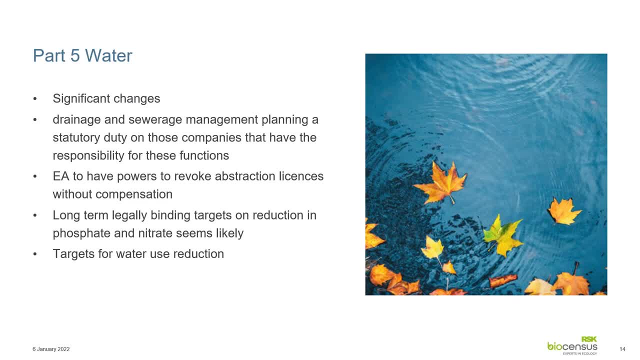 table amendments. throughout the passage of the bill, which I'll come on to in a sec, as mentioned previously, there's been justified criticism of the amount of sewage that is legally- believe it or not- discharged, as well as, obviously, the illegal discharges. I think personally this is a great example of where the 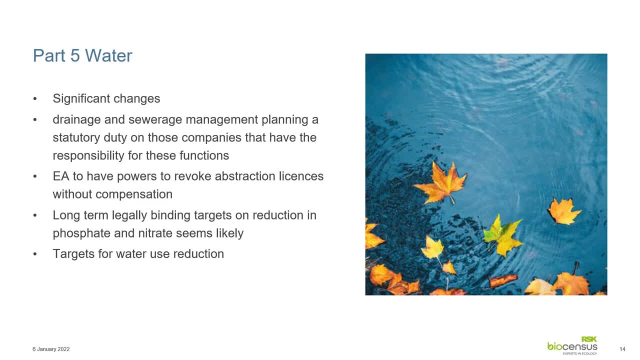 current system really isn't fit for purpose. the legislative framework we have at the moment allows this to happen and it just seems wrong. the big one here is that the Act will make drainage and sewage management planning a statutory duty on those companies that have the responsibility for these functions. another significant change is in the 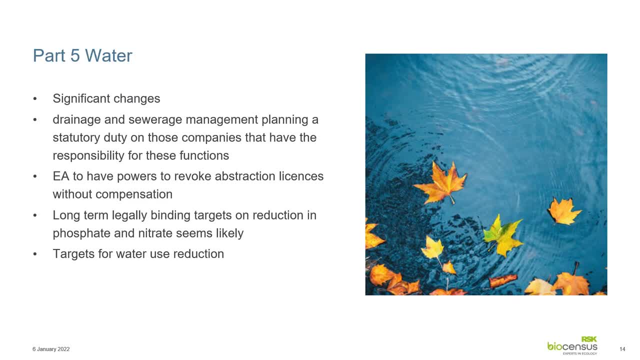 ability of the Environment Agency to revoke obstruction licenses without compensation, even for long established rights. however, it would appear that these changes would be more effective if the environment agency were to revoke the policies that would be in force until 2028, going back to long-term binding targets for water. it would appear that the 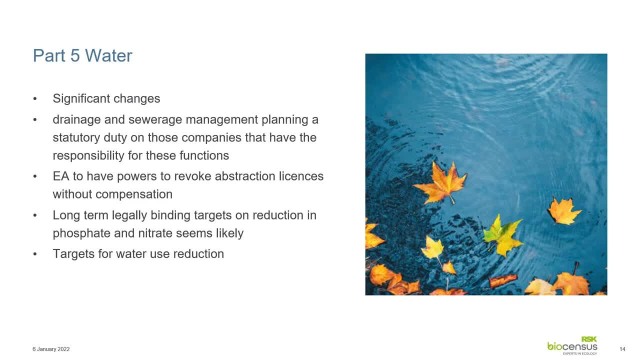 reduction in phosphate and nitrate loading are to be targeted. I think those are joining us today that are building houses anywhere near SPAs in water catchments. won't be surprised by this, and the direction of travel by a lot of policy has been very much in this direction anyway. further to this there: 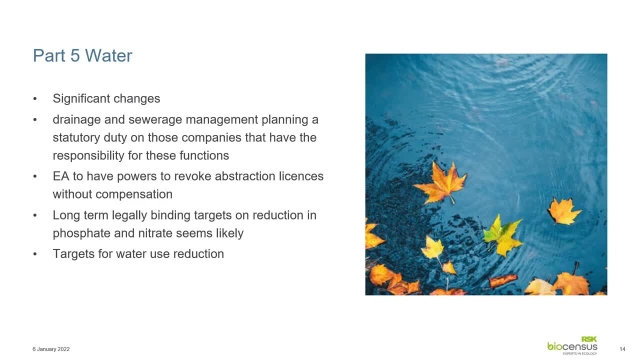 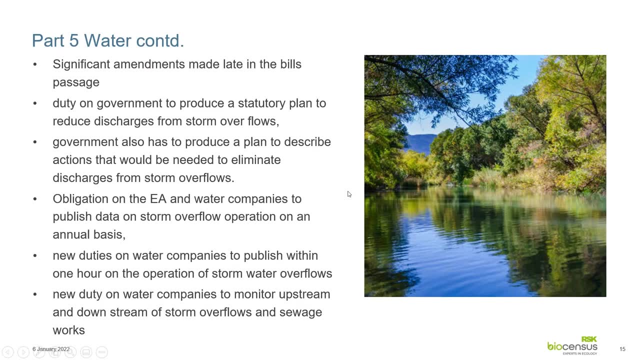 will be targets set for the reduction in water use and demand, which presumably has added benefits such as a drastic reduction in carbon use. during the passage of the bill- and I'll talk about the amendments now- there was an amendment tabled by Philip Dunn, along with a few others and, as a result, some 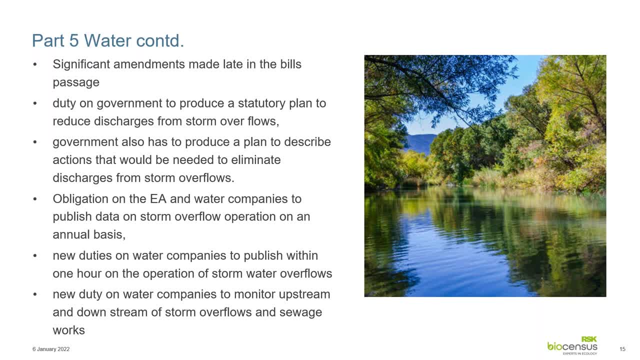 truly significant changes were made to the draft bill. these included a new duty on government to produce a statutory plan to reduce discharges from storm overflows. government also has to produce a plan to describe actions that would be needed to eliminate debt, as it were, death neuen. 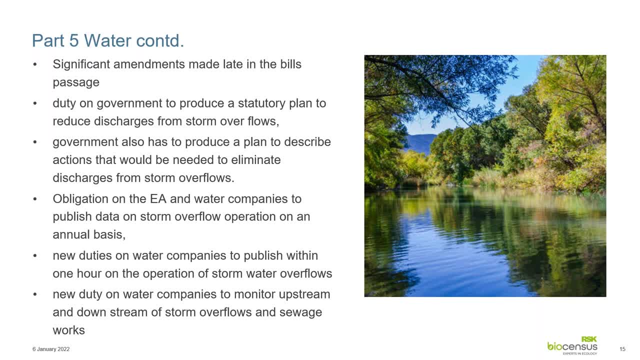 discharges from storm overflows. furthermore, there will be an obligation on the environment agency and water companies to publish data on storm overflow operation on an annual basis and new duties on water companies to publish within one hour on the operation of storm water overflows and a new duty. 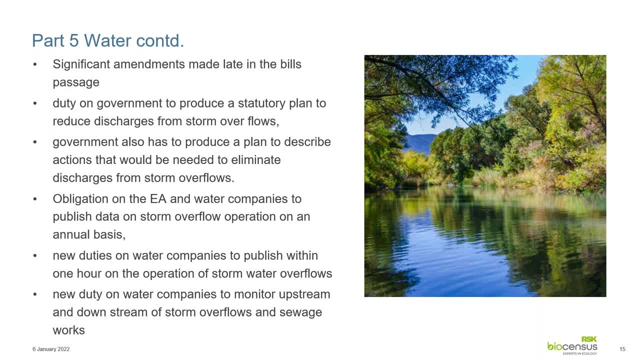 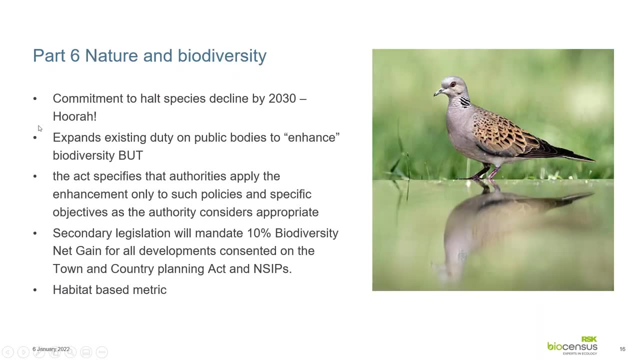 on water companies to monitor upstream and downstream of storm overflows and sewage works. I must admit I wasn't aware that that wasn't already being done and it seems a bit bizarre that it wasn't great that it's in the Act. Okay, part six, nature and biodiversity, and you'll forgive me for dwelling a bit. 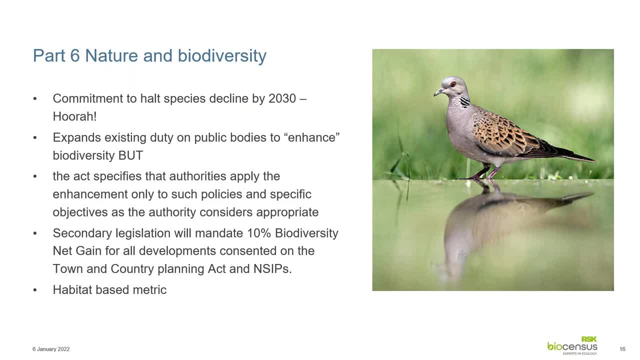 more on this than some of the other areas, but sure you'll understand why. The headline here is that the Act commits to halting species decline by 2030.. Big cheers This has been, and I'll try and remove the cynicism from my voice, but this has. 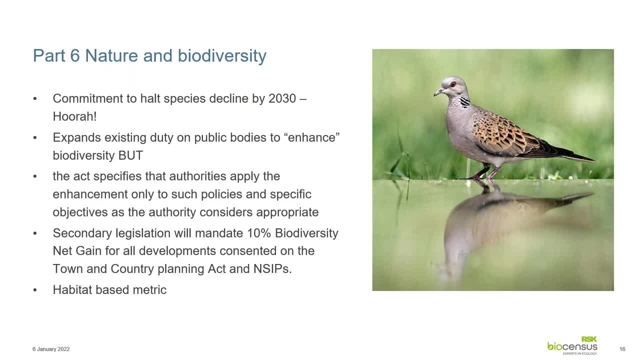 been a massive win for the Act, and I guess the devil is always in the detail and we have heard about these sort of targets before from various organizations across the world. but you know, it's a great point to start with and an ambition On the face of it. the Act expands the existing duty for public 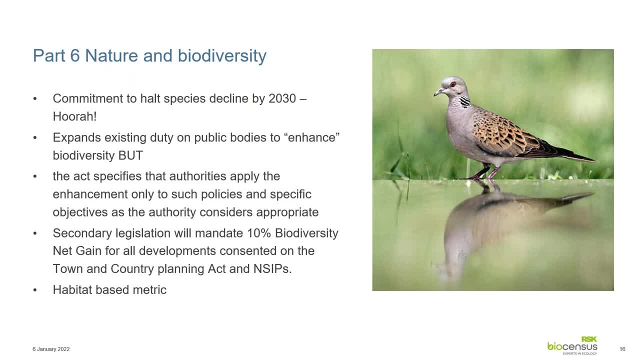 authorities to ask sorry, by asking that they enhance biodiversity. this enhancement, or net gain, is a common thread running through a lot of policy and NGO rhetoric at the moment and, let's face it, if this Act is going to achieve its objective of leaving the environment in a better state than that, 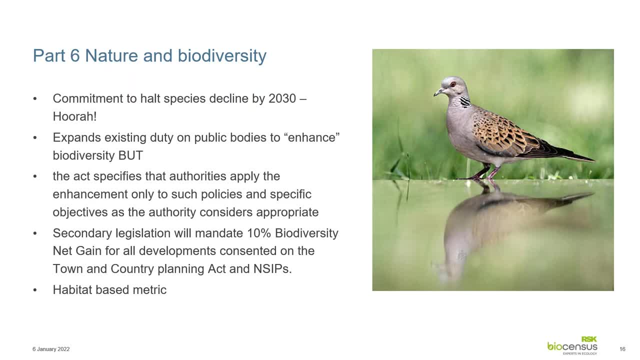 which we found it. net gain is the only way forward. One slight issue is that the Act specifies that authorities apply the enhancement only to such policies and specific objectives as the authority considers appropriate. To me, that's another warning sign. Something to watch. The language is a bit too loose, I think, from my personal point of view. 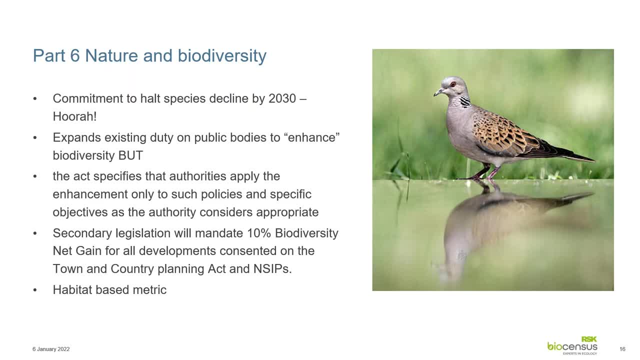 Okay, so biodiversity net gain: This is much talked about element of the Act. and well, at least in the ecological consultancy world, The Act is going to mandate, through secondary legislation, a requirement of all developments consented under the Town and Country Planning Act and those of 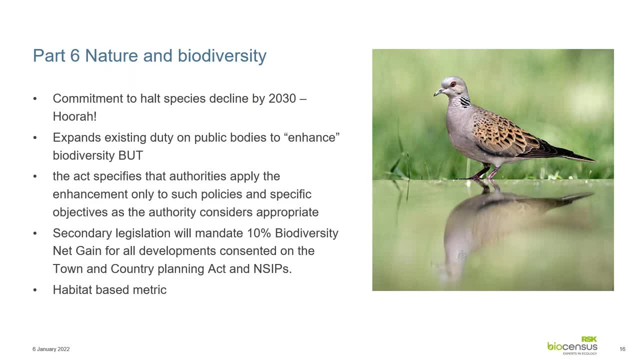 nationally significant infrastructure projects, pretty much all developments. a requirement to produce and demonstrate a 10% net gain in biodiversity value. For the first time, these will be legally binding agreements and some of which may be delivered through conservation covenants, which I will talk about. 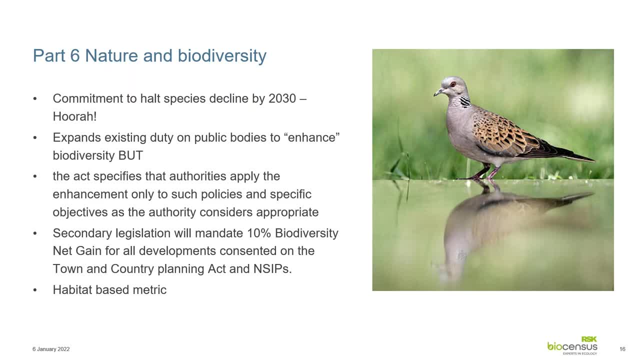 in a minute. I think that from here, there's going to be a step change in the way all schemes- from from small hands, builders of two or three homes, all the way through to master planning for new towns- there's going to be a step change in the way that this is approached with a view. 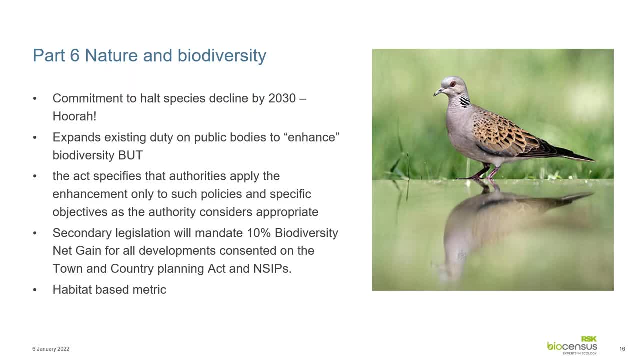 to enhancement. The calculation of the principle of enhancement is key to leaving the country in a better state than which we found it. The measurement of biodiversity is currently done via an assessment of habitat and, again, there has been much debate over whether this is a good metric to 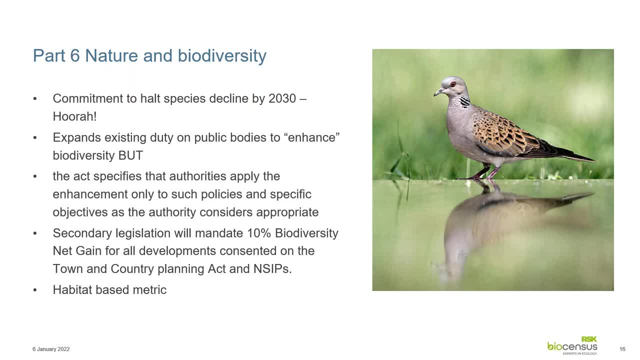 use. One thing is clear, though, I think, is that it's clear and it's transparent and there's a level playing field, which I think is important from the industry adoption point of view and, to be honest, let's face it, anything that was going to try and assess biodiversity value was always going to be. 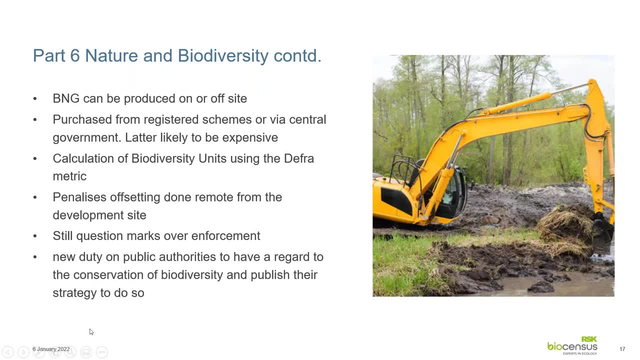 up for debate. there will be various options open to developers, from on-site gain through to offsetting via registered schemes or by purchasing from government. it's likely that this last option will prove expensive and therefore i think we're predicting an emerging market in habitat banks and 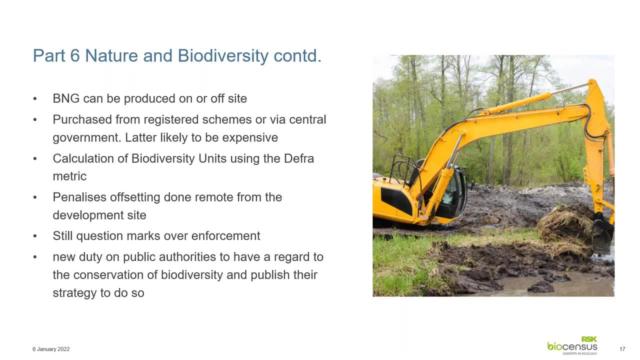 other landowners offering their land as areas for biodiversity enhancement and, to a certain extent, we've already seen movement in this area. currently, the defra metric- we're on version three at the moment- penalizes offsetting of schemes that are geographically removed from the development. 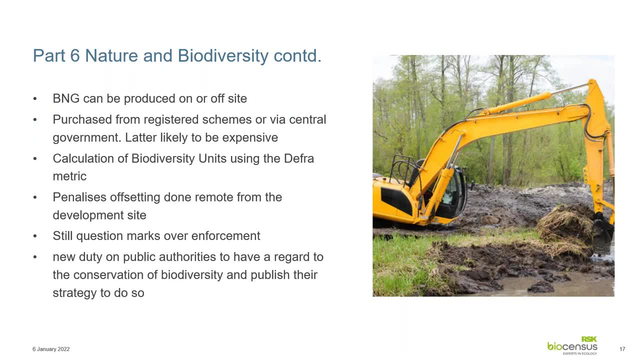 the idea is to prevent people offsetting miles away from where they're doing the works and making their offset less relevant to that particular impact. at the moment, if you want to offset off your site within the local authority where you're operating and you have, say, the need to offset 10 units- biodiversity units- then that you will have to find 10 units within. 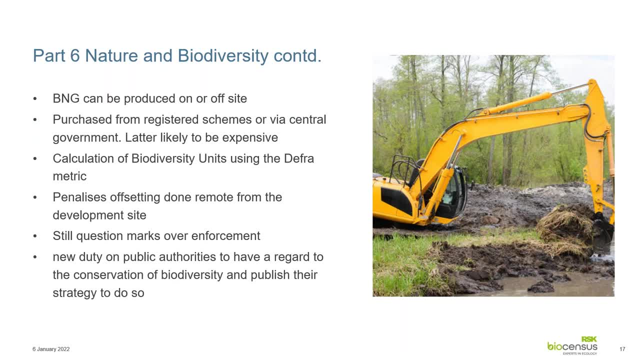 that local authority. if you go to the authority that's neighboring to next door to where you're doing the works, then you will have to multiply that by 0.75, so your 10 units become 15.. if you go further away than the neighboring one, all the way up to miles and miles away up in north scotland or 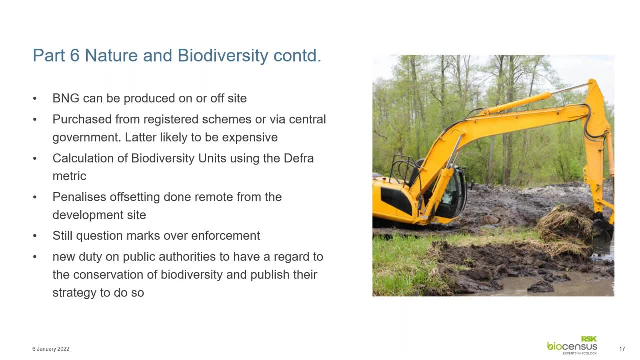 you have to multiply your need by 0.5, so your 10 becomes 20.. my personal view is that the economics of land prices and the differential between, say, the north of scotland or the isle of moore compared to essex or kent or somewhere in the southeast would mean that actually it. 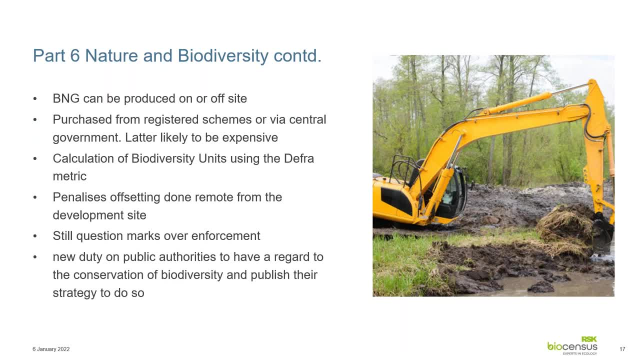 still might be worth offsetting further north. so i my personal view, is that we'll have to change in order to maintain the principle that the offset is as appropriate and as local as it can be. so i want to say that i've been working on it for about 15 years now, so i'm going to 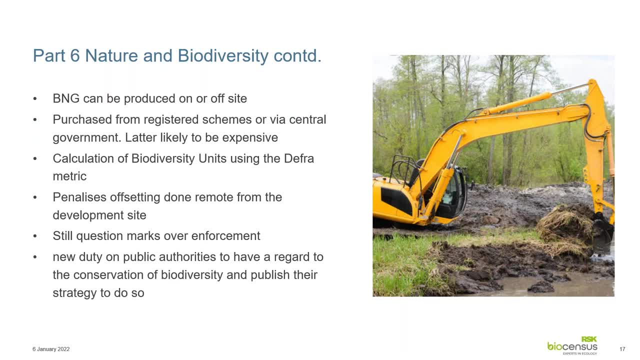 do a little bit of a close up on that and then i'll come back to it, but i'd like to have you and me and our staff to sort of go over it as we think about the future of the process. there is, however, very little resource currently within the local planning authorities to 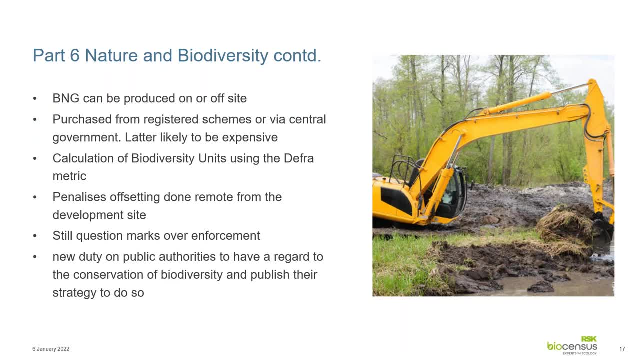 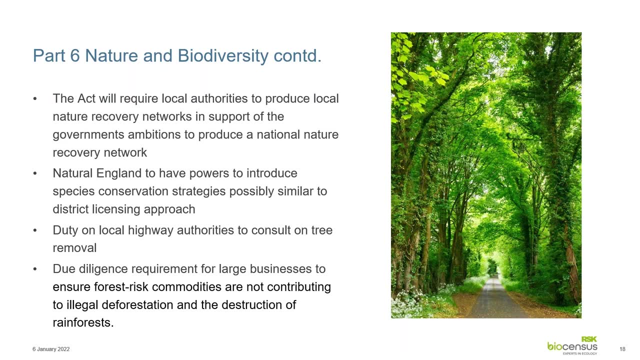 effectively enforce their statutory requirements as it is they have currently. i mean one in three local authorities have an ecologist. i would worry that they're going to have the capacity to enforce this and report on their plans to do so. Further to this, a key element of the Act, 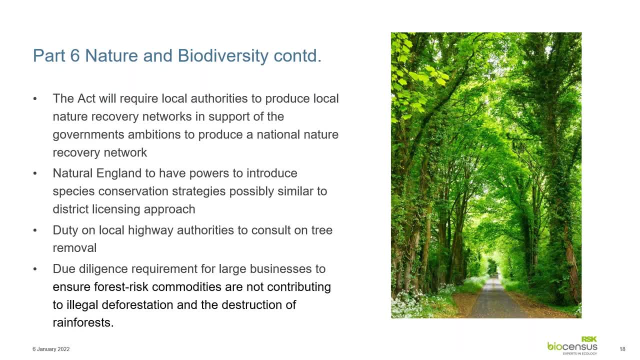 is to require local authorities to produce local nature recovery networks in support of the government's ambitions to create national nature recovery networks. It will insist that local authorities will have regard to these strategies. How this will be reviewed and assessed is still not clear, but the 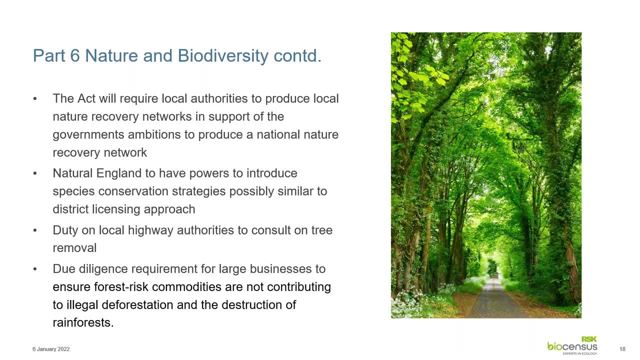 principle is one of more strategic approach to species and habitat conservation. The so-called laughtonian principles will apply, but bigger, better and more joined up. An area that's still fairly unclear is that around the remit and powers of Natural England. According to the text of the Act, Natural England will have powers. 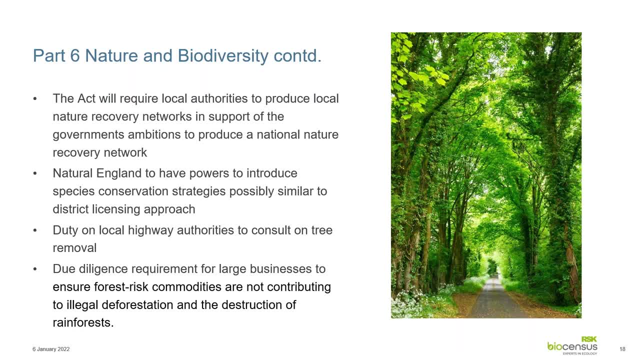 to introduce species conservation strategies, for example, and these would be similar to district licensing approach, although the details of this remain unclear For those of you that live in field. there was also- you might be interested to hear- that there's also a duty on local highway authorities to consult with local communities before felling street trees. we also see here. 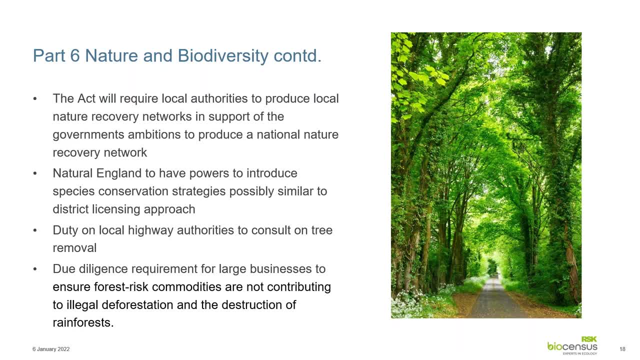 a tacit acknowledgement that we don't protect the world by being an island, and this is, i think, quite a significant piece of the legislation and maybe a marker. it isn't going to solve the whole problem, but it's a marker and a good start in my view. but there is a new due diligence duty for large. 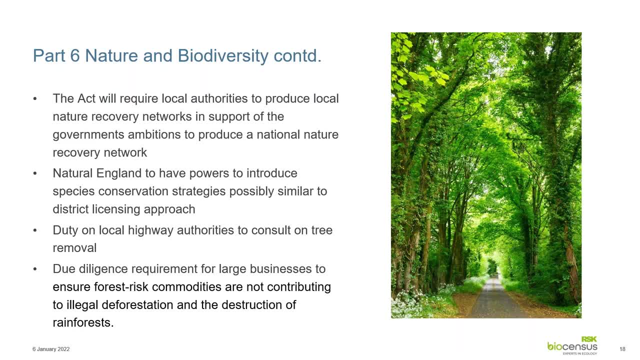 businesses to ensure forest risk commodities are not contributing to illegal deforestation and the destruction of rainforests. a cynic might, if you were speaking to one, point out that much of the world's deforestation isn't actually illegal and that most of the deforestation is happening legally within that country. but it's still deforestation. but i guess. 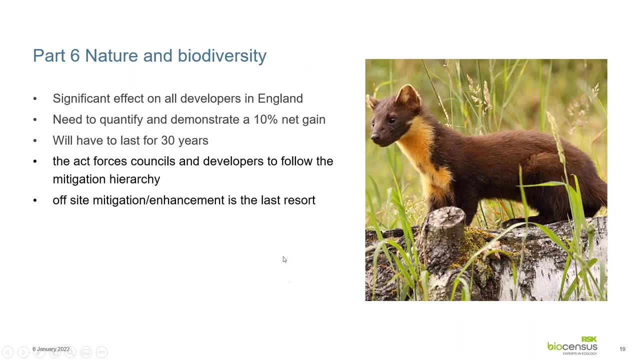 like i said, this is a start and something that probably should be welcomed and built on. so how will this affect developments in england? the act is going to have a significant effect on all developers in england and possibly northern ireland. all developers will have to. 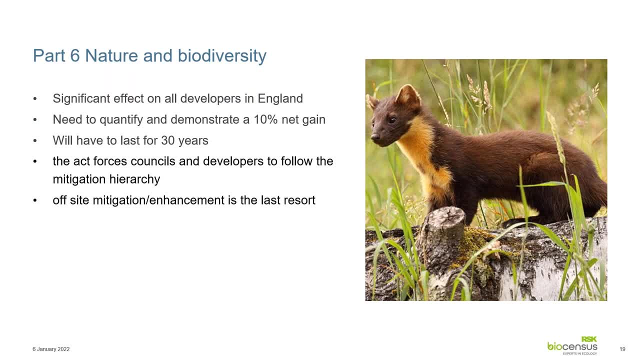 show how they are going to achieve a net gain of biodiversity as a result of their scheme, but not only that, but demonstrate that this game will exist for at least 30 years. i don't think this is going to be easily achieved and you know, i'm not sure many developers of 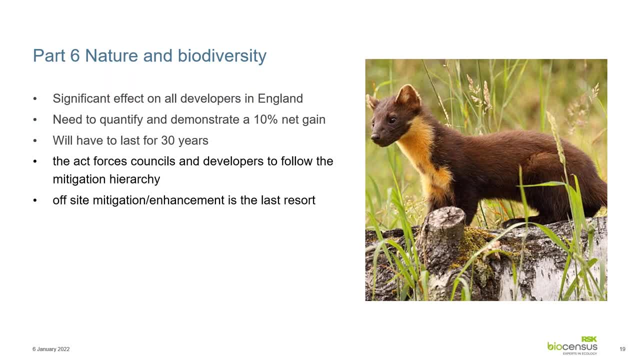 house builders, or even large tier one contractors, are going to want a liability of 30 years or less as a result of this, and i think it's important that we keep this in mind. one option is conservation covenants, which i'll mention in a minute, but it's probably worth. 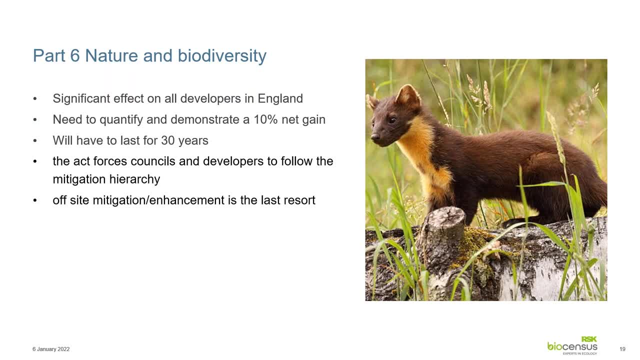 pointing out that most permitted developments and small householder applications are going to be exempt from the biodiversity net gain. a significant change from the point of view of an ecologist is the act forces councils and developers to follow the mitigation hierarchy, although in practice this is already followed. the basic premise of offsite mitigation enhancement is: 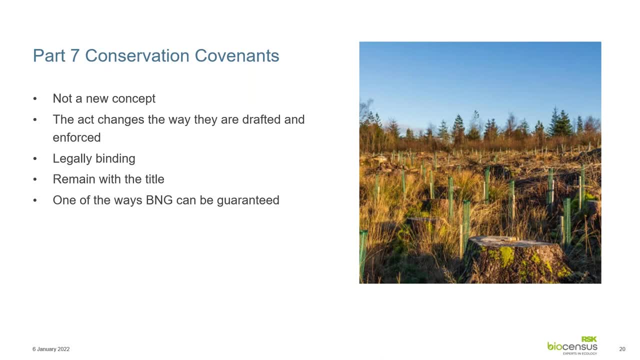 So conservation covenants- I'm just going to briefly talk about this. they're not a new thing. they've been in place for quite a while, certainly if you've been operating in and around SACs in the south of England. there is many conservation covenants applied to homes when you buy them. 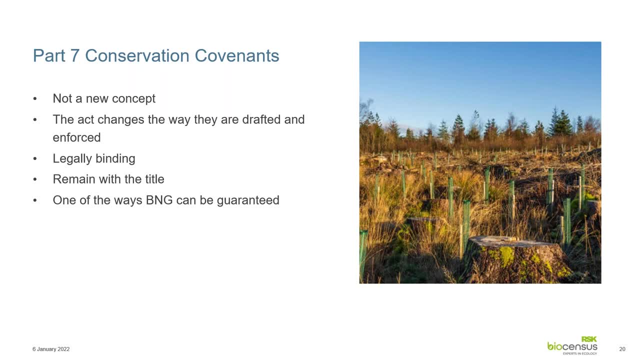 The difference here is that the Act sets out specific ways that these will be enforced and ensure that all conservation covenants will be voluntary but legally binding, and that's a big difference. In addition, the covenant applies to the freehold, the title of the land. therefore, 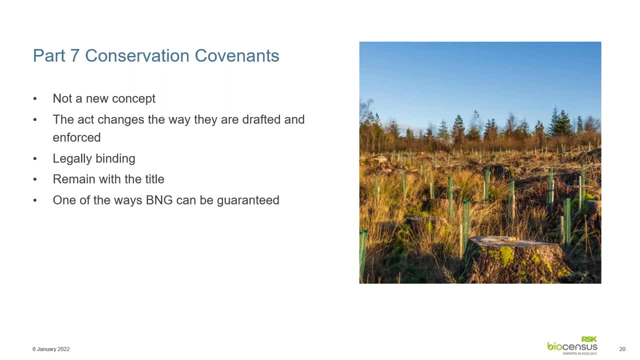 will be passed on through sales as opposed to being applied to the individual. Of course, there is an intrinsic link here between conservation covenants and biodiversity net gain, and the covenants are just one way that biodiversity net gain can be achieved for the long term. 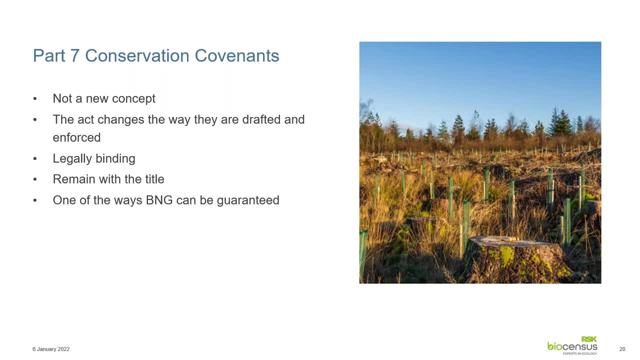 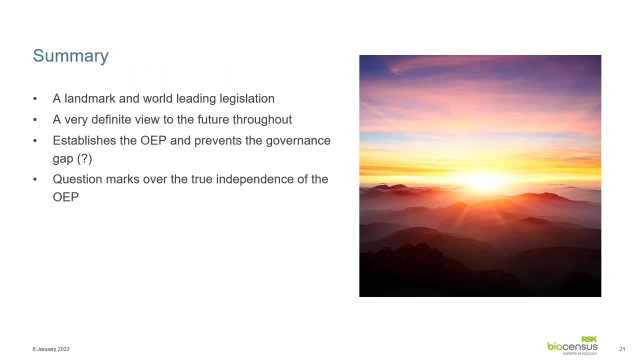 Again, this reference is running through the Act for the long term. My final point here is to say that this is brand new, not tested, legislation. Any view of its value and the consequences is, to a certain extent, always going to be an exercise in crystal ball gazing. 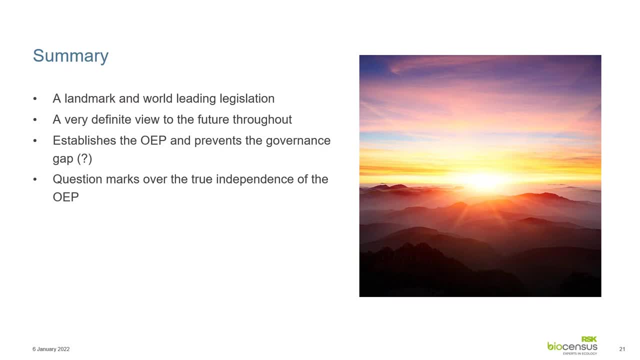 I, for one, will be watching the inevitable test in case law that comes from this with great interest. The government has referred to the bill as a landmark and world-leading legislation that will transform how we protect and enhance our environment. It sets out a comprehensive and world-leading vision of conservation covenants and biodiversity net gain, and the covenants are just one way that conservation covenants and biodiversity net gain can be achieved for the long term. There is an absolute need to see more covenants and biodiversity net gain as an evidence of sustainability. 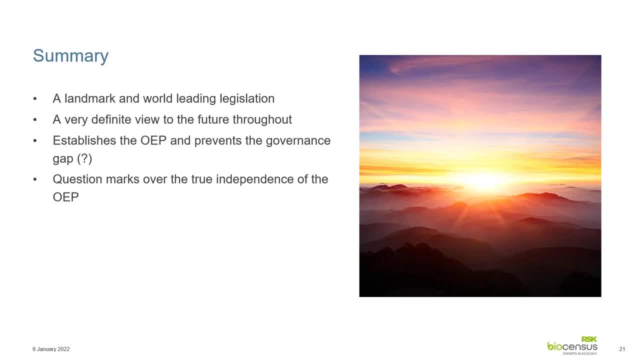 but it's also needed to have a very clear vision to allow our environment to prosper and for the future generations, and to ensure that we enhance and maintain our environmental protections. There is a clear sense here of longevity, of a long-term view and strategy, For someone that has observed too. 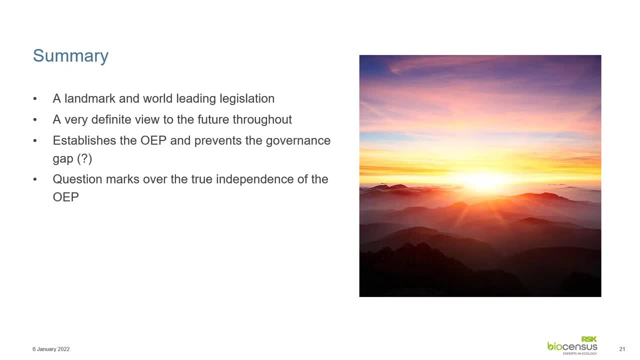 many environmental policies with too short a time view. this is welcomed. Again, however, we must ensure that the pressure to deliver is high into the long grass when it becomes politically expedient to do so. the establishment of the oep is arguably the most significant consequence of this act: whether it will have the independence 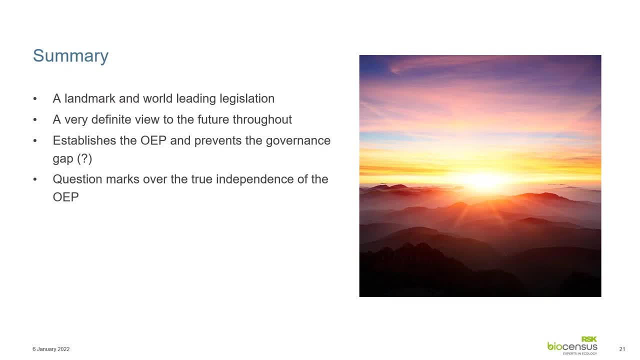 and teeth that mr gove imagined remains to be seen. as i said at the start, this situation represents both a huge risk, as we leave the governance of the european court. at the same time, a huge opportunity, a once-in-a-generation opportunity- to develop a truly world-leading framework for 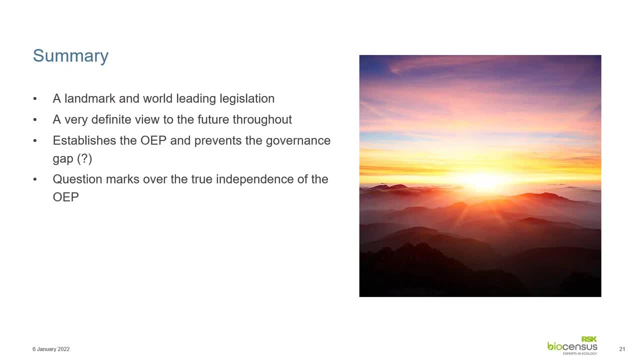 the management, protection and enhancement of the environment. there is currently some justified concerns that, despite the rhetoric, that there is still a governance gap in our environmental protections post-brexit and certainly not having recourse to a higher independent authority worries me. i guess time will tell if this is truly a landmark and world-leading piece of legislation. 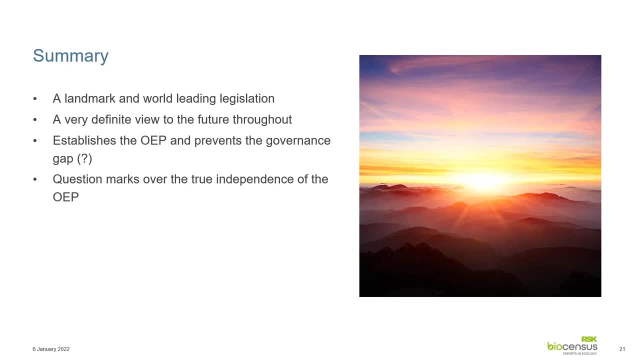 and whether or not it will be the case in the future. I guess time will tell if this is truly a landmark and world-leading piece of legislation and whether or not it will be the case in the future years to come. we'll look back on this time as the time we made the big positive step to reverse. 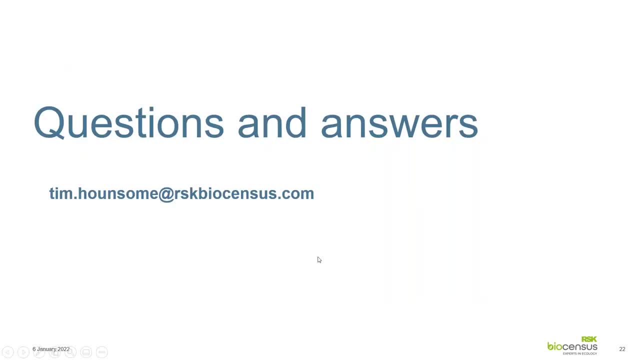 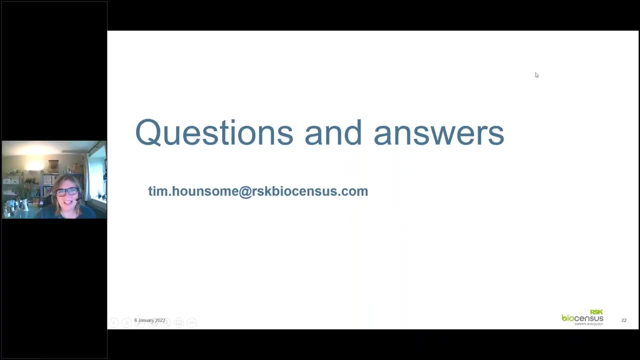 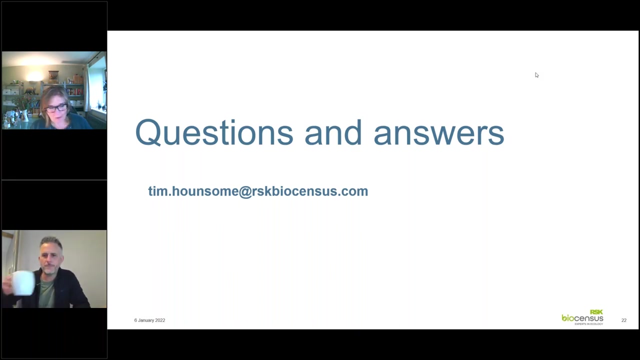 forever the damage that we had done. thank you very much when i'll take? thank you very much, tim. excellent, can we see you again there. we are perfect. um well, we've got quite a few questions and not very many minutes left, so i'm not going to get all of them in, i'm afraid, and 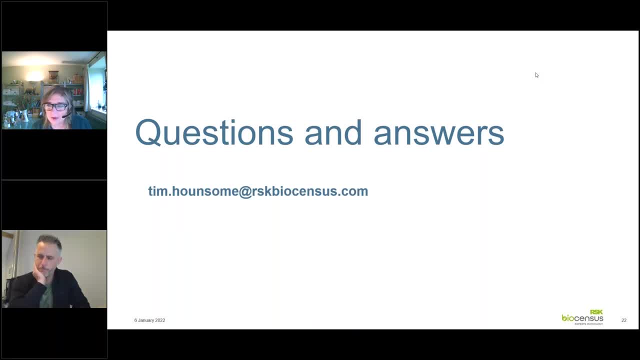 we will try to answer any of them separately afterwards, but if i could just ask you a couple first of all, um, we've got a question around. you've given us a good review of what's in the act. uh, what's missing? is there anything that you would have hoped to see in the act, or that's not made? 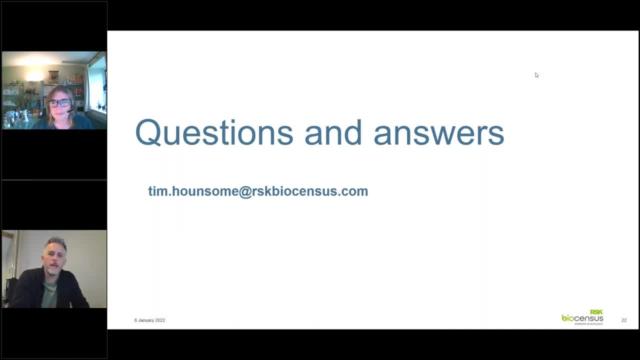 it at all or that's been lost in the drafting. i guess that's inevitably there, always will be, and everybody would have a personal view on that. um, i think one of the ones that stood out for me was the um, fairly weak might. one might say um. 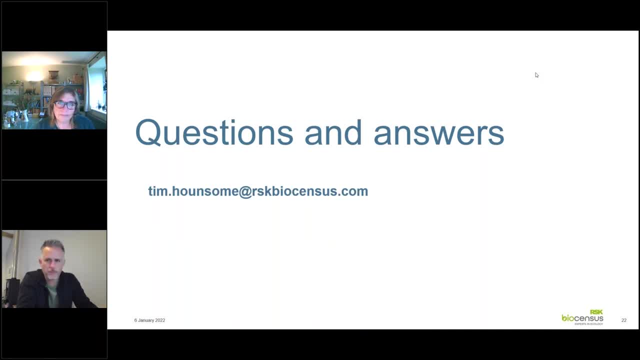 um clauses on on the use of plastic and the how we were going to deal with with waste and with plastics. um, i think at the moment just having a- you know, take your bottle back and get 10p back, or whatever it's going to be that we used to do as kids- um, that doesn't seem to really tackle it, and 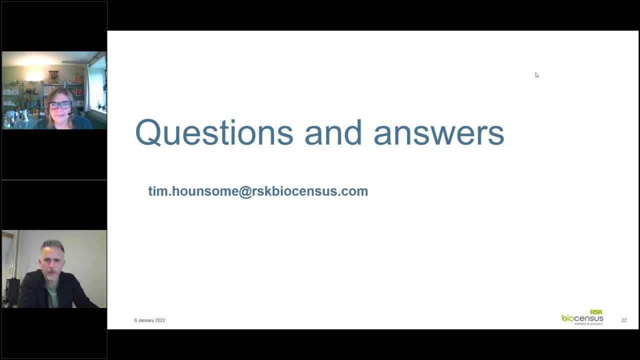 you know, i noticed that recently our prime minister said that recycling didn't work. um, so i think having those two things combined worried me a little bit. um, i think having, to a certain extent, it was always going to be the case, but i think having the lack of teeth and um independence of the oep is yet to be proven. 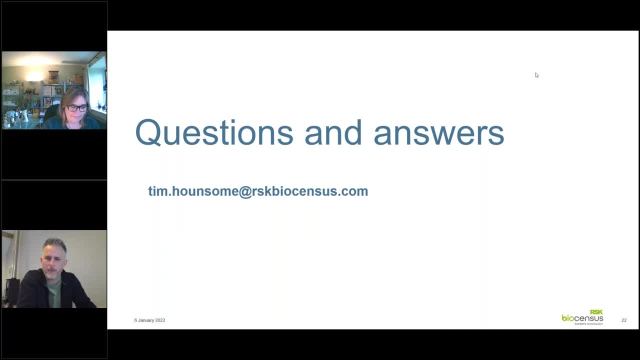 and i know that everybody thinks it will be okay. but at the moment i think the funding of it is um direct government, of central government, and so i do worry that it might end up being a little bit stuck, the same way that maybe you know some of the sncos have been in the past. 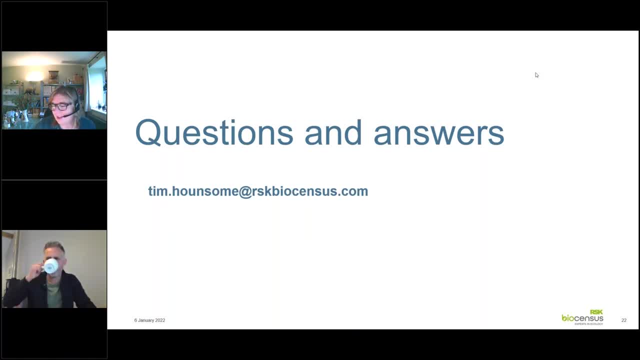 absolutely, yeah, i agree, and um, i'm also old enough to remember bottle recycling- though they were glass bottles in those days- um, but yeah, nothing, nothing on microplastics really is there, or vehicle tires and so on. so, yeah, i, i think i'd agree with with those areas. um, i got another question around. 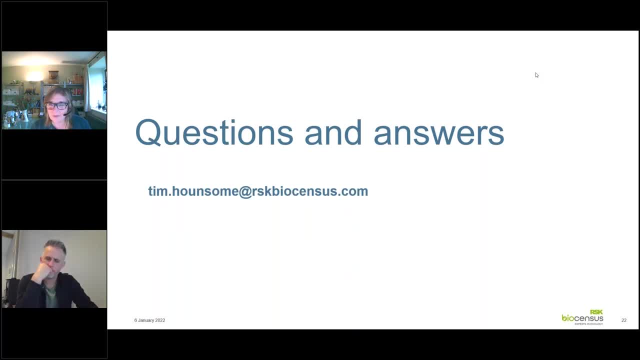 um, you know, as ecologists, most of the time we're talking about things like the wildlife and countryside act um is. is the wildlife and countryside act affected in any way by the environment act and are we expecting any changes there to things like protected species legislation? yeah, good question, um, i think the quick answer there is that the environment act has no, no. 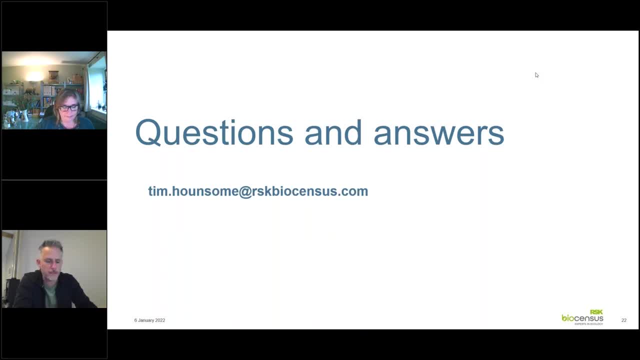 influence on the wildlife kind of side, that that legislation is still there and still still enacted and being being used. um, i think, from an ecologist point of view and a conservation point of view, um, i would like to see further legislation, or at least revised legislation, for the wildlife and 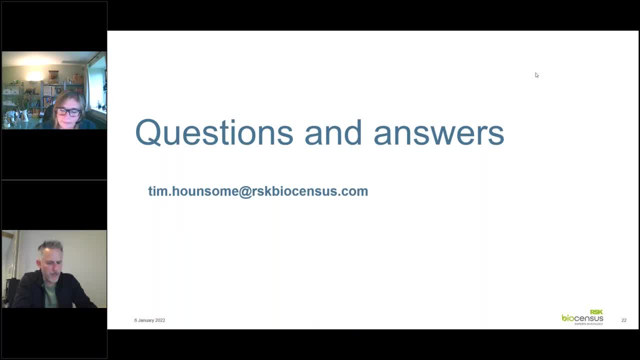 countryside act. i think when i talked earlier about some of our current protections and legislation being not fit for purpose anymore, i am largely thinking about the wildlife and countryside act, and the obvious thing to pick on here is the schedules of protected species that largely stuck in the mud. there's lots of, obviously, i know about birds and there's lots of birds on. 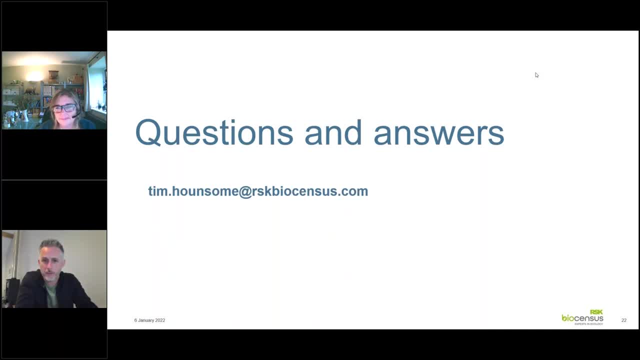 that list that shouldn't be on it potentially- and there's certainly lots of birds that aren't on it. that should be so i think revising the wildlife and countryside act is going to be the next sort of cap off the rank from my point of view, and i know that there's a quinn: i need all review. 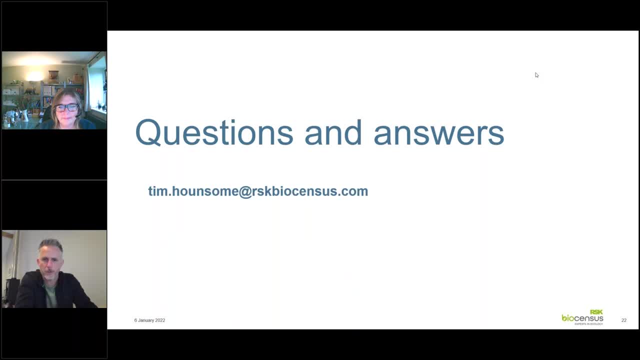 that's taken place and that's going to be in consultation soon. but i think that's that we, if we can dovetail in a fit for purpose, modern, dynamic, um, wildlife and species protection legislation that dovetails in with the environment act, and then that would be a really powerful piece. 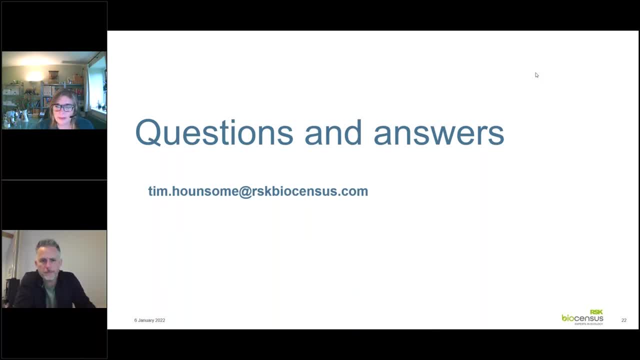 of dual legislation. thank you very much. um, i've probably got time for one or two quick ones. um, i've got a quick one here. um, when does the 10 net gain for biodiversity requirement actually kick in? and and a kind of related one, if you like to that. 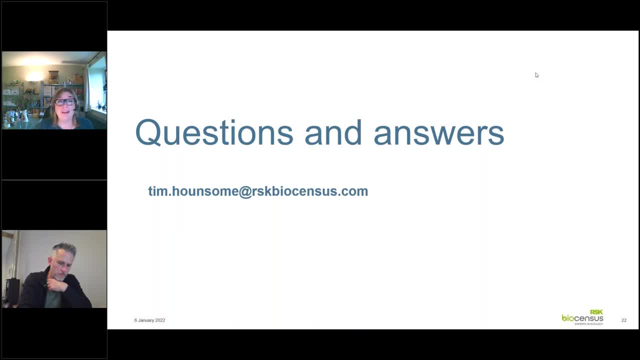 um who will make the judgment that 10 gain has actually been achieved? good question um the net gain. the management net gain is going to rely on secondary legislation, so so to a certain extent the timetable is is dictated by that, but i think i'm right in saying. 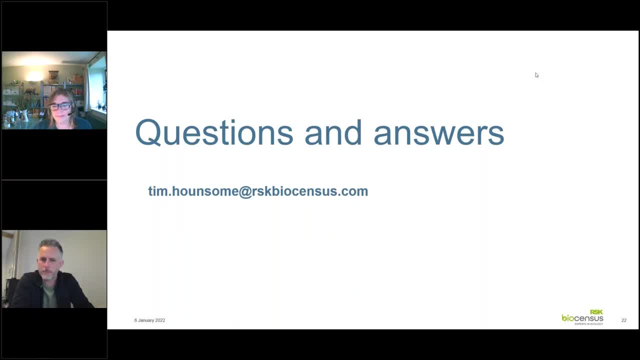 and stuff. you probably know better than me, um, that we're going to be looking at 18 months from now, so that sort of timeline, yeah. but who judges this? at the moment? it's going to be down to the local consenting authority. but, as i said in in my tour, the resource to enforce that and to 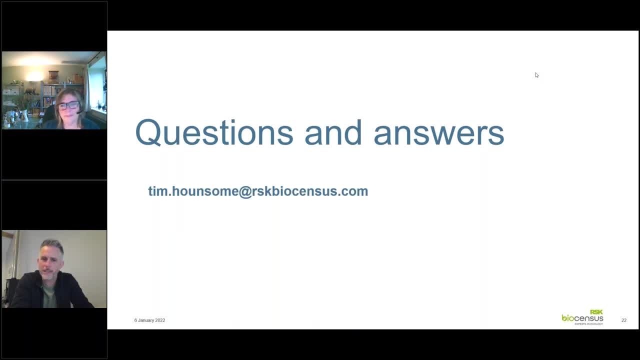 monitor it? um, almost certainly isn't there. so i think there is a bit of a gap and a bit of a worrying gap there with how this is going to be played out. i'm confident it will be resourced and it will, and it will be that sort of gap will be closed, but at the moment we're still sort of second.